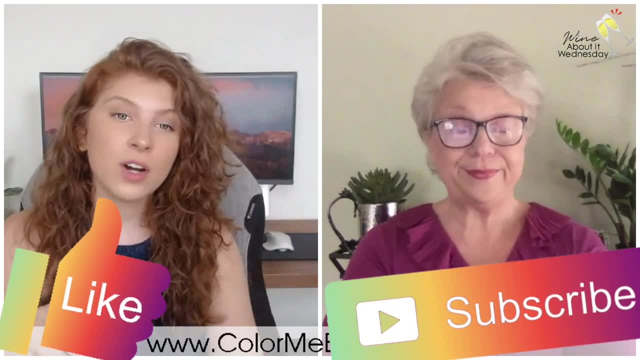 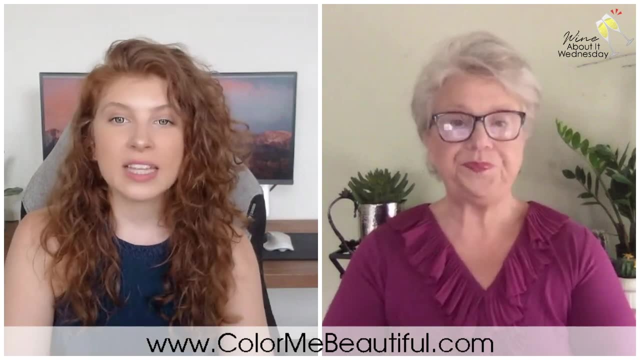 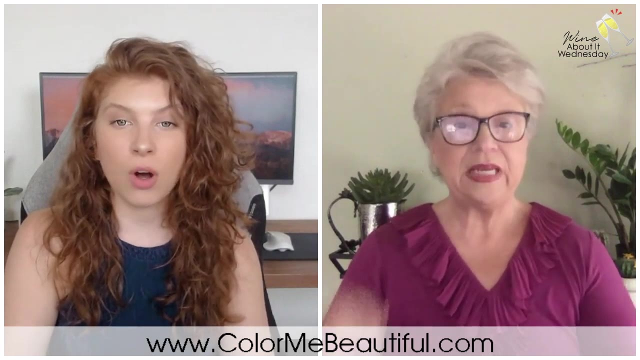 you can impress people with. So I know, a little while ago you gave a tip on how to look at patterns and kind of see what the overall theme was And you mentioned- yeah, you kind of mentioned- making your vision a little blurry-eyed towards the pattern and kind of getting the overall color. 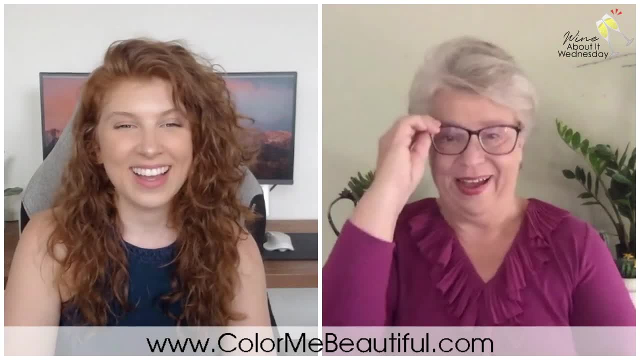 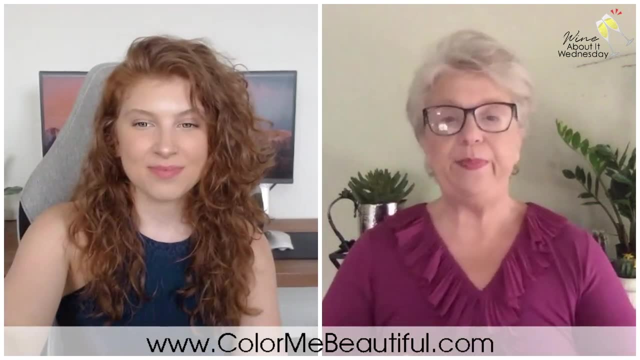 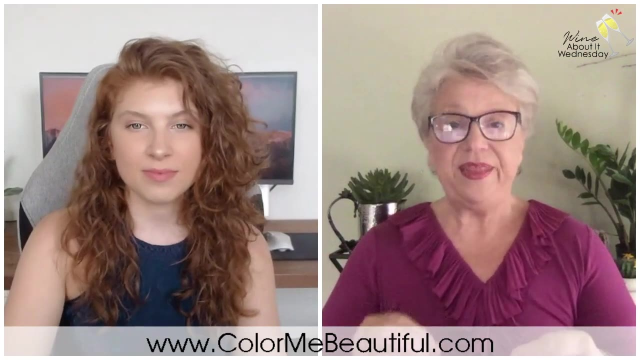 Like this: Well, there you go, It's super easy for you, But it's more than that. I mean, that was kind of a quick little tip, but it's a little more complicated than that, because each season has its own characteristics that you need to embrace as much as you say: oh, I'm a winter. 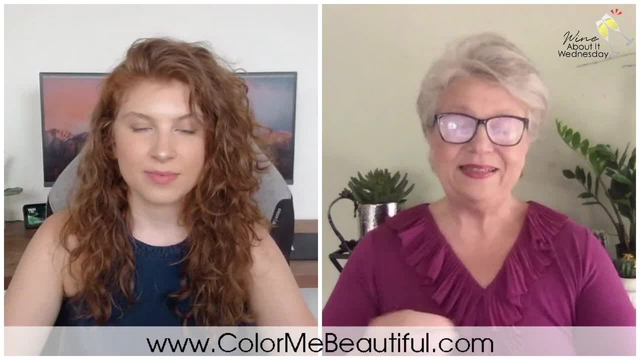 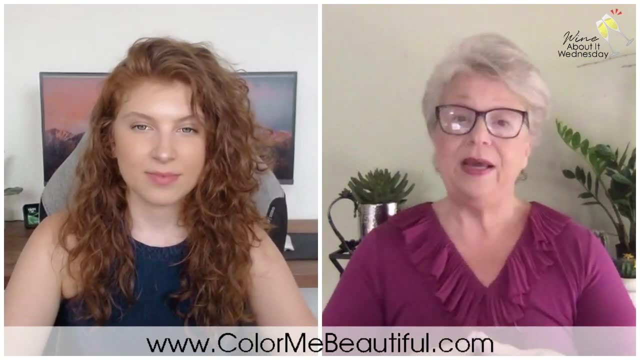 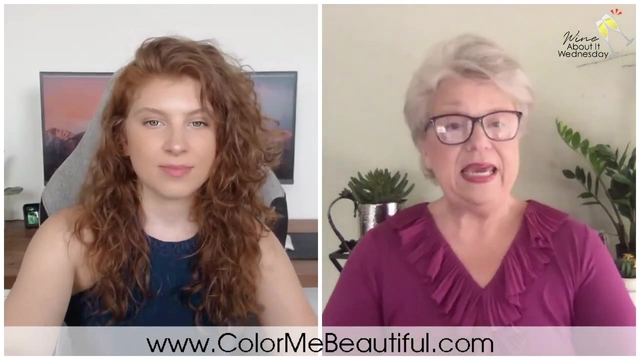 or I'm a summer. There are certain characteristics that you must embrace along with your season. For example, if you're a winter, you must also learn that you're clear and high contrast, high contrast and cool. And if you're an autumn, you must learn that you are soft and warm, like Sarah. 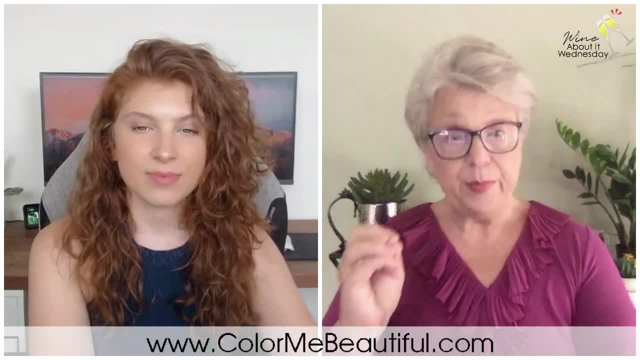 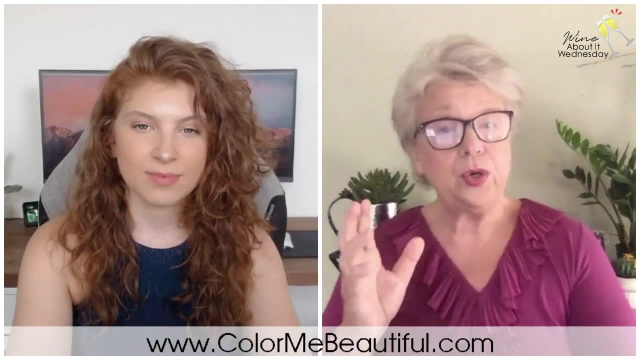 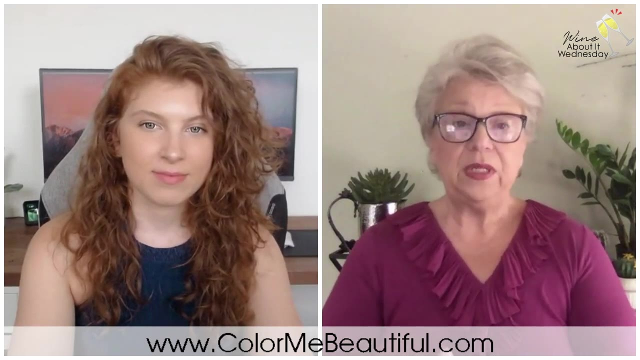 soft and warm. If you're a summer, you need to learn that you're somewhat powerful. If you're a winter, you need to learn that you're powdery, you're muted and you're cool, And if you're spring, you need to learn that you're warm and bright, And this will help. 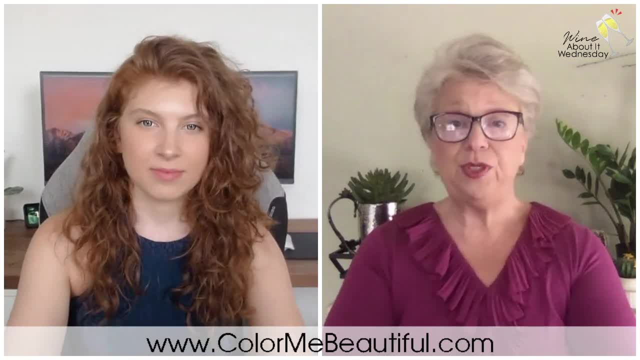 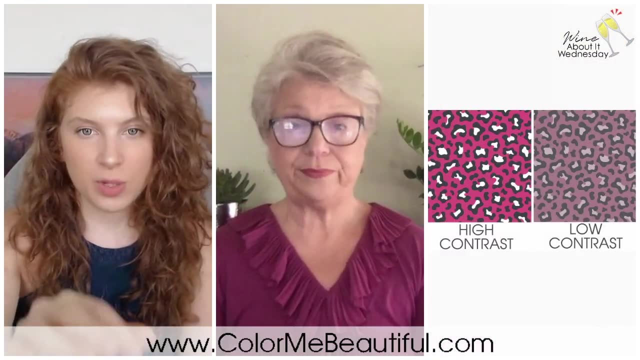 you choose your patterns moving forward and you'll be able to do it like a pro. So I guess I should probably bring up those slides for us just to visualize. So when you're talking about winter and summer, we have winter on the left and summer on the right. 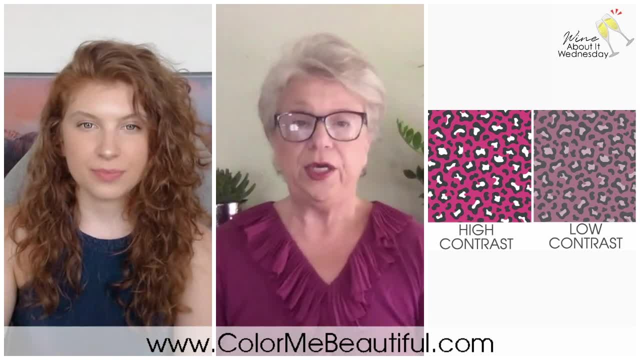 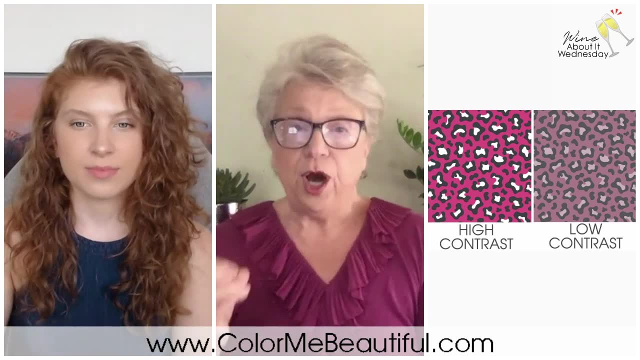 So imagine, if you're in winter, You have summer, You have winter, You have winter And you're able to choose your pattern under different conditions. You have a lot of these patterns and you have a lot of different trends You have. I think you're going to hear me speak. 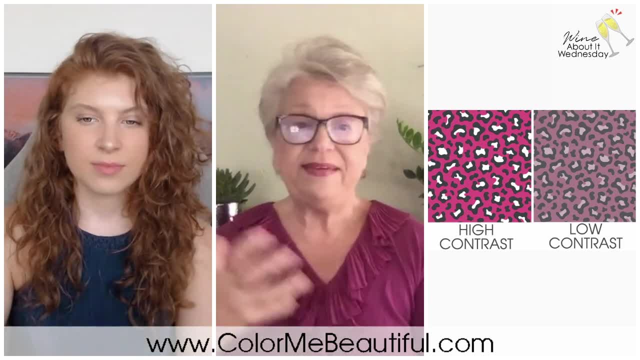 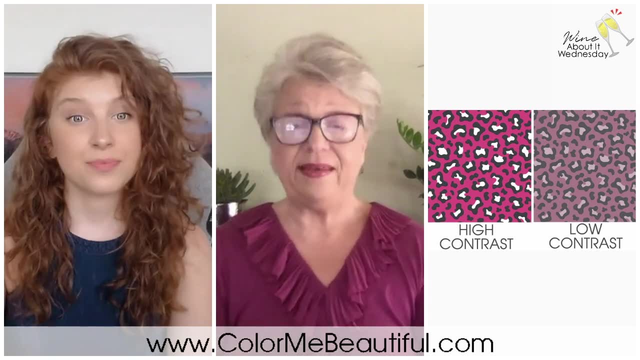 about this a lot. But you have a lot of these patterns that you come up with. You have your pattern that you have black hair with no red or gold highlights. You have dark brown hair, no red or gold highlights. So the contrast in its heat, the dark hair, the contrast between 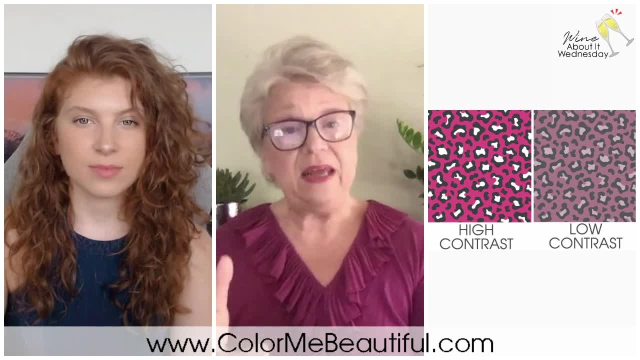 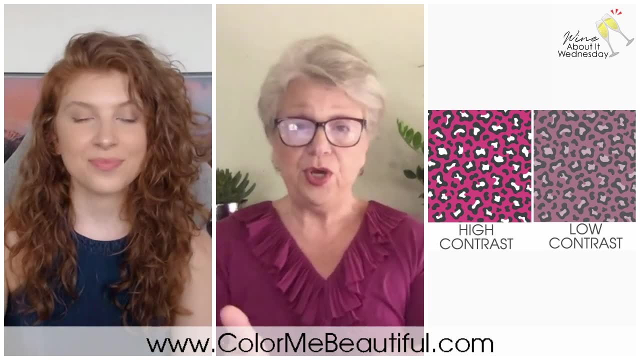 your hair and your skin tone. that has high contrast and of course, you know- all of you know, if you tune in with us regularly- that if you're wet or you're a cool season, so as you're looking at these patterns, you look for something that's got cool colors in it and you look for 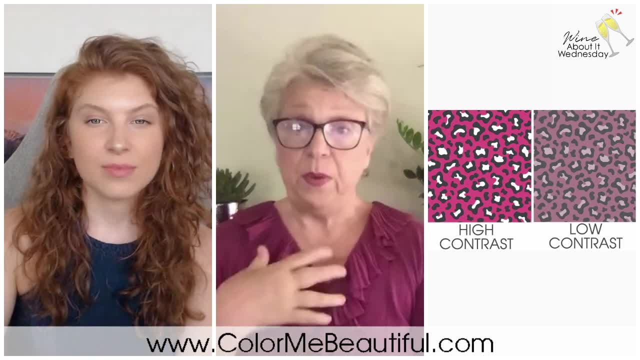 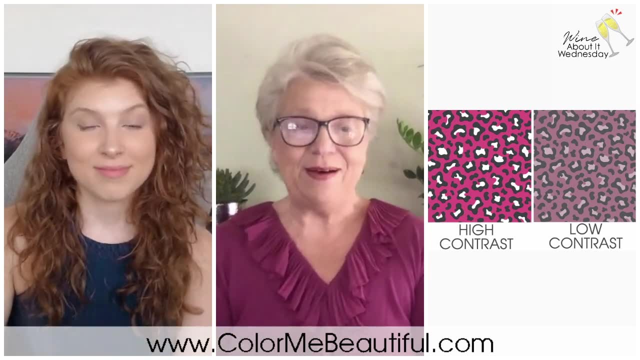 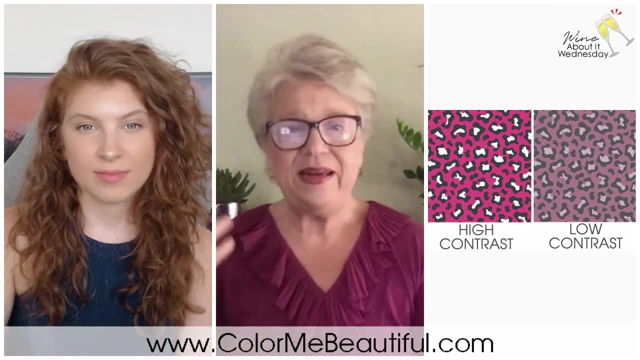 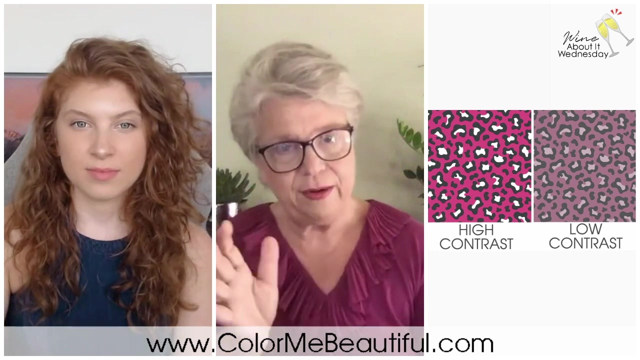 something that's got high contrast. and then for someone like me, if I'm looking for a mask or whatever of wild, I'm gonna look for low contrast, because if you look at the contrast between my hair and my face and it's all kind of not contrast, it's just kind of muted altogether. 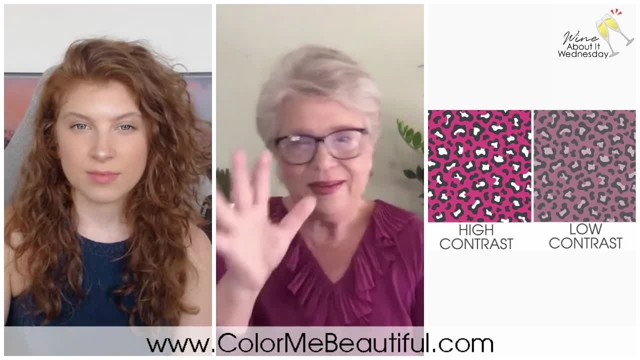 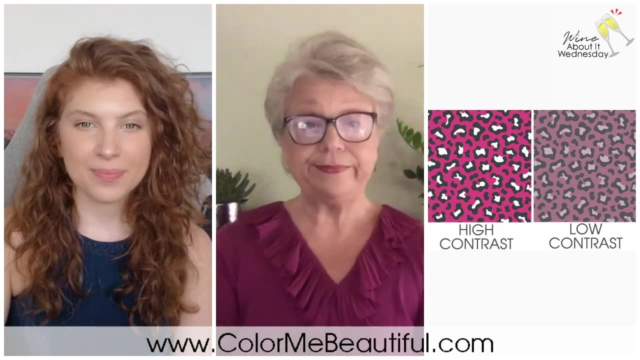 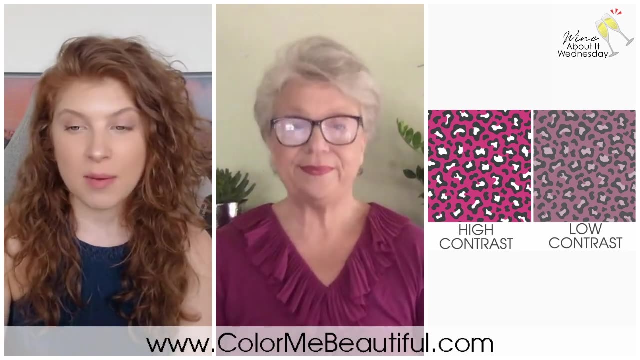 you like to say it's grayish, grayish. so I'm gonna look for, as a summer, a low, something that's cool. so just one last time: our high contrast is the winter, which is on the left, and our low contrast is the summer which is on the 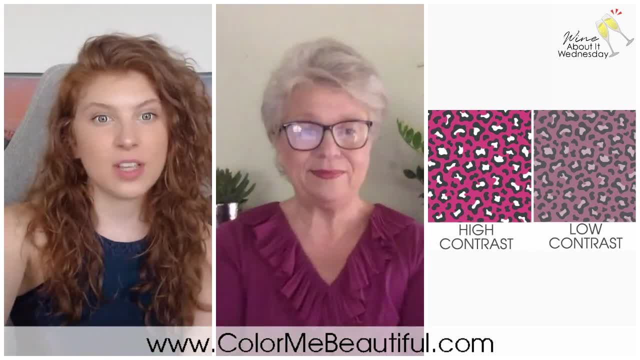 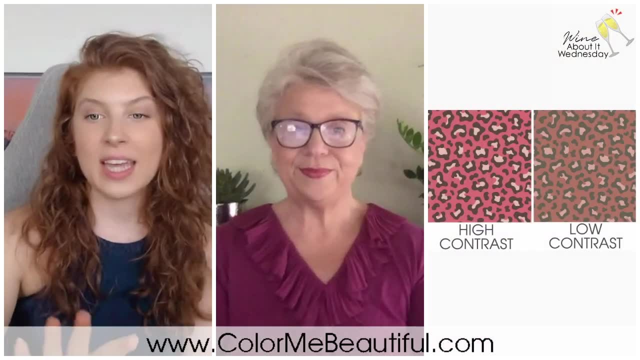 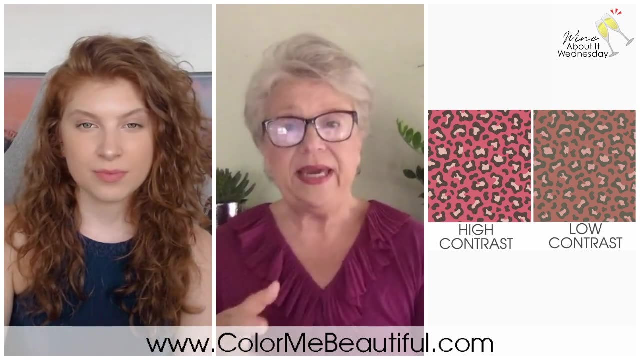 right, and both the different them are cool. yes, both of these are very cool. now let's check out what happens to the warmer seasons. so now we're gonna bring up spring and autumn. okay, now I call this high contrast, but with the spring, your, I like to say right, spring. 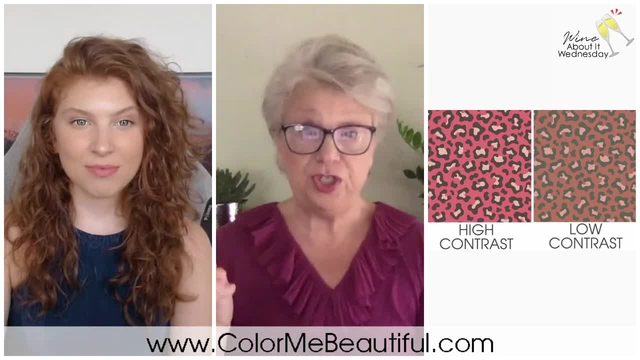 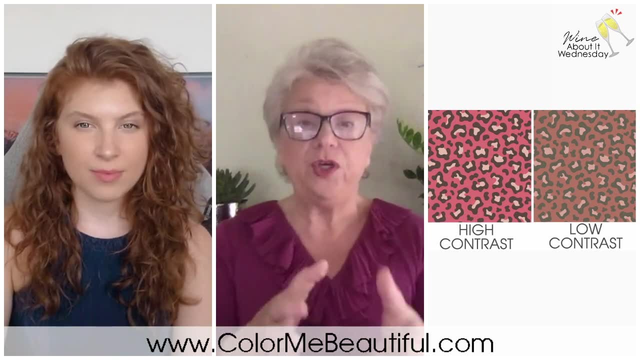 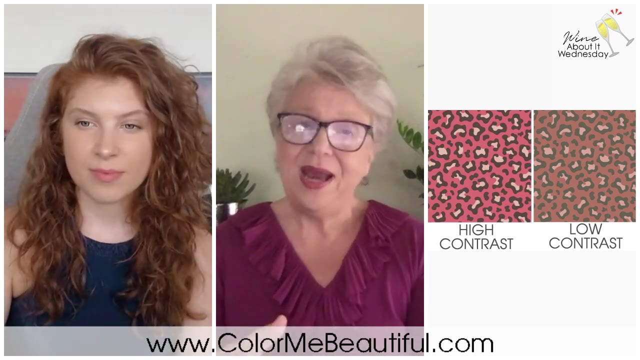 it is my contrast, contrast here than the autumn, which is soft, but I like, I like to call it right because the spring, even though it's warm, your choices are brighter. they're, they're more colorful than the autumn choices, which are not not colorful, they're just lower. in contrast, they're more muted, they're. 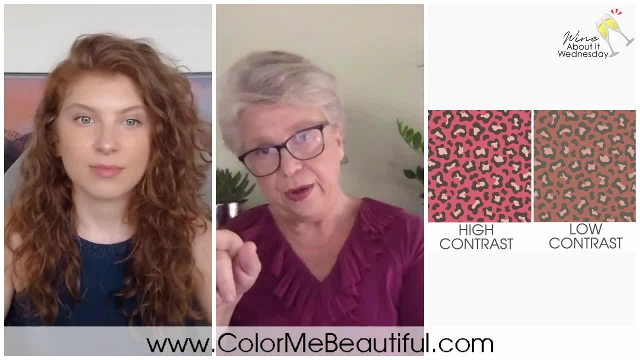 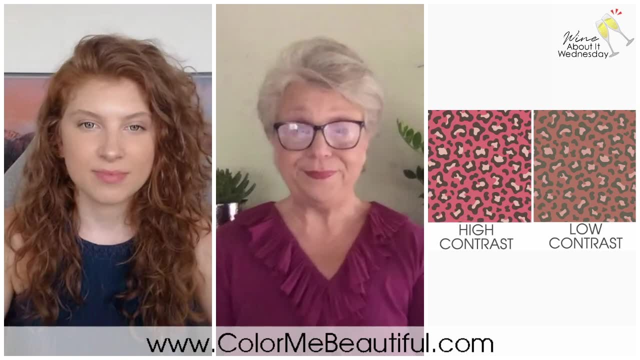 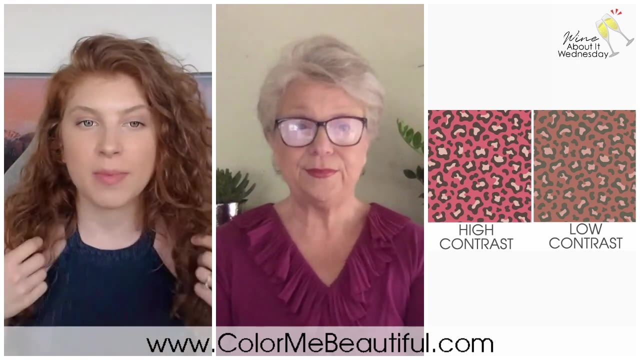 softer. and if you look at Sarah and then look at this low contrast slide, you see that that's kind of indicative of what the per right right remember. the goal is to harmonize the entire look together so that low contrast really harmonizes with my hair color, with my 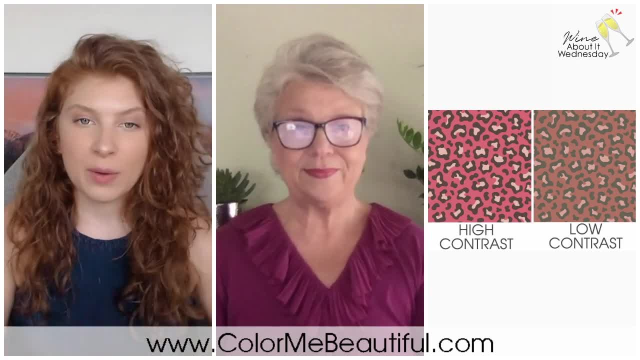 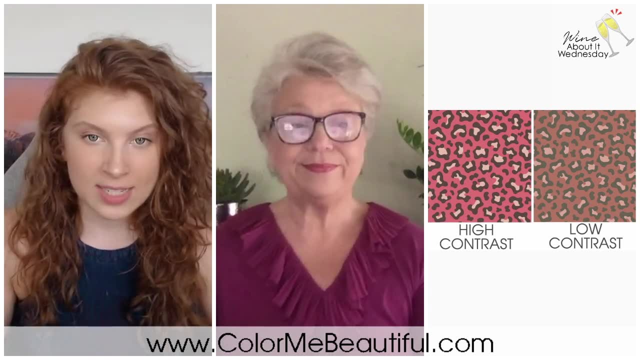 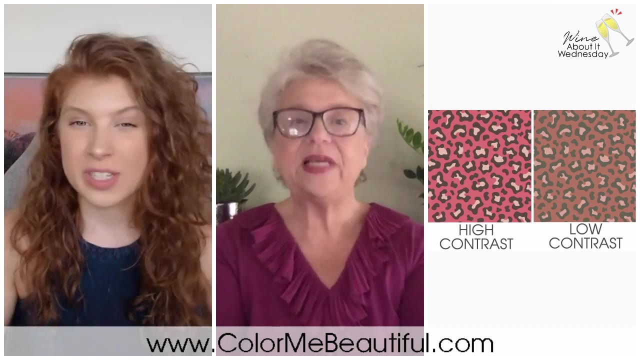 eyes, with my skin tone and it also being warm. now I want to mention one last time: on the left we have our spring, which is high contrast, and on the right we have our autumn, which is low contrast, and then both of these are warm season. so you have that warm pink for the almost coral or salmon, or all salmon, yeah, on. 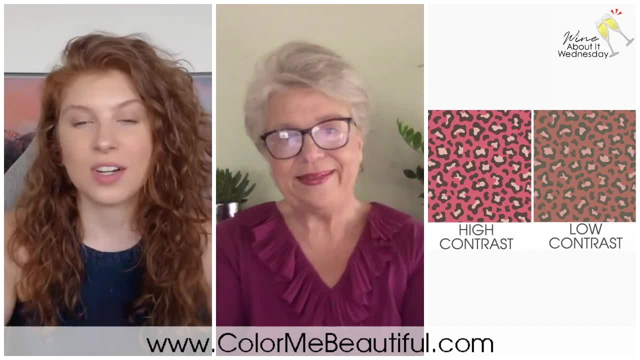 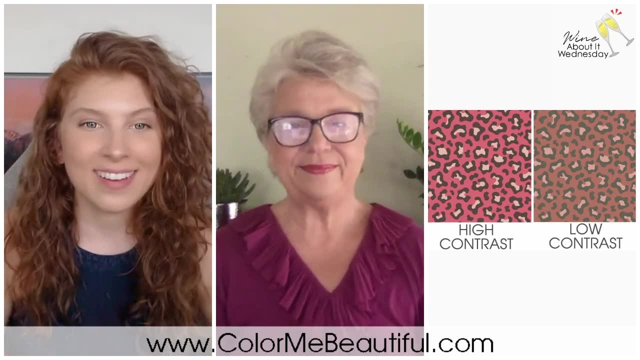 the spring side. and then you have that rust terracotta color on the right favorite, which is gorgeous. I love it. I could wear that in green all day long, I know. so I want to make sure everyone that has the chance to look at these two slides. 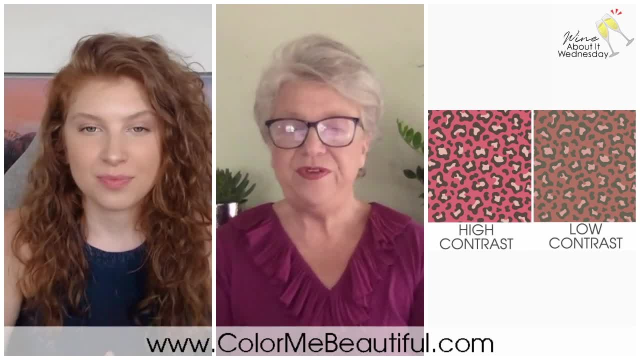 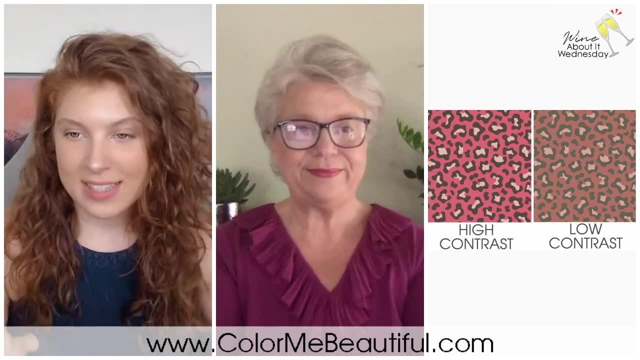 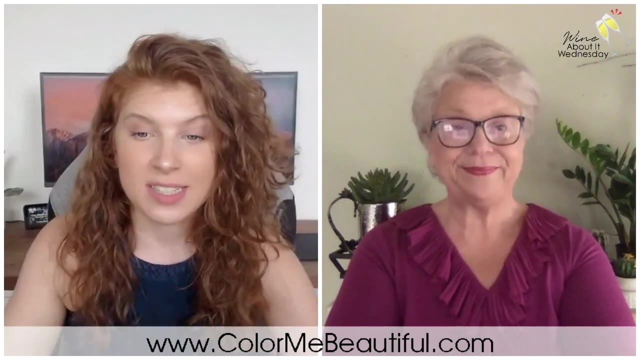 just to kind of get the visual. and for you professionals among us, those of you who are color analysts, as always we make these available to you at no charge. of course, I will leave them in the comments down below when we hop off, but let's move on to looking at different patterns for this season. so I think the first 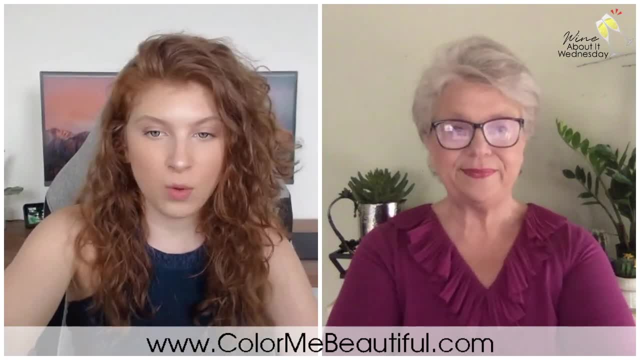 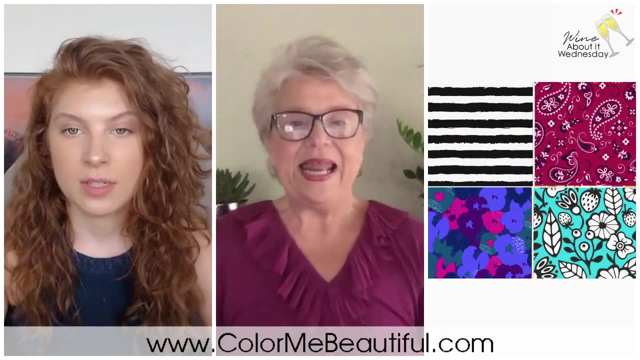 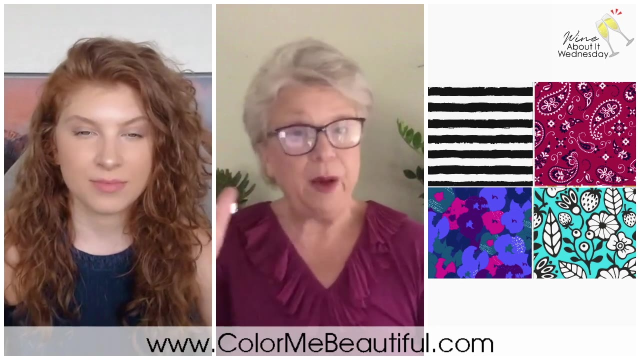 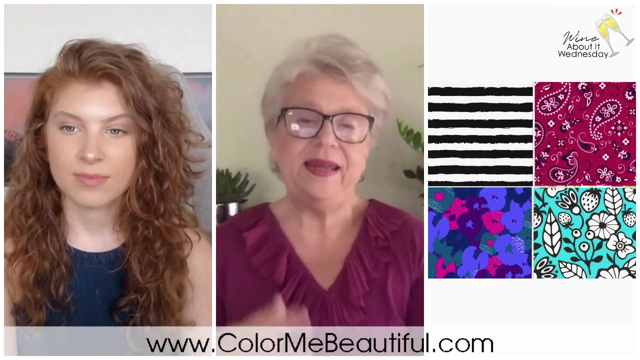 one we did was a winter, so let me grab the winter for us to take a look at now. these are gonna be patterns and textures that are strictly winters, and I had great fun putting these together because I got to shop in my mind for those friends and family that I know who are winters in doing so, and I have to tell. 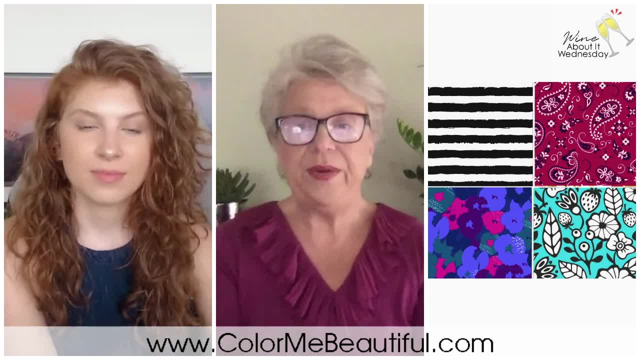 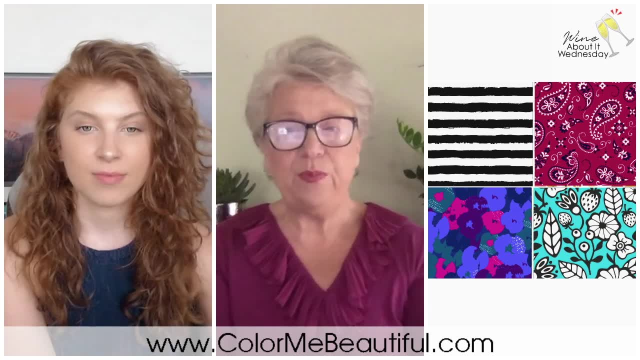 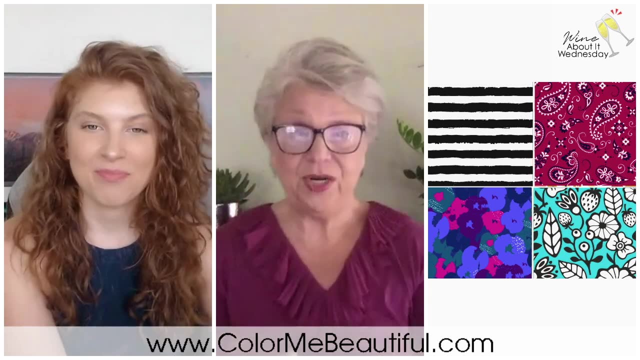 you. I'm playing around with the mask idea in my mind. you know what would. what's new here? our winters. one of the classic winter combinations that they can pull off, that nobody else can, is the black and white, a black and white pattern at any time, and that is very contrast, high contrast and an ideal for the winter. 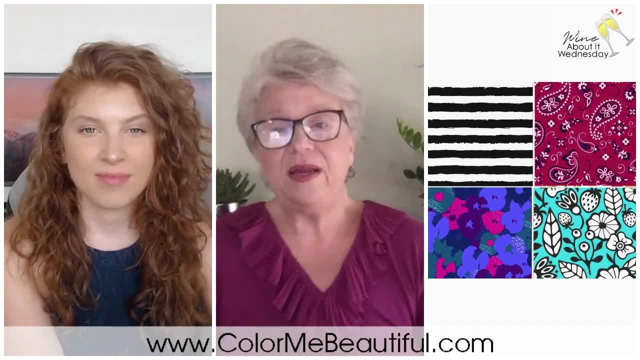 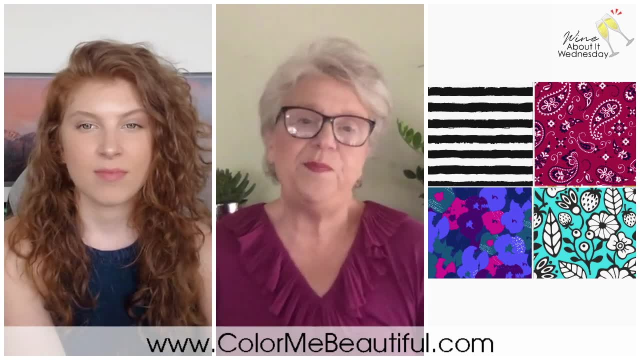 season and as I was looking at that, I thought, okay, so what about bandana? if I were choosing a bandana for a winter person? and I went with this berry, and I know that it's a good color, and it's a good color, and it's a good color and it's. 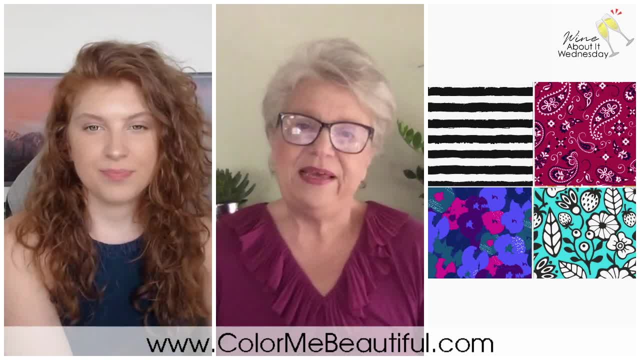 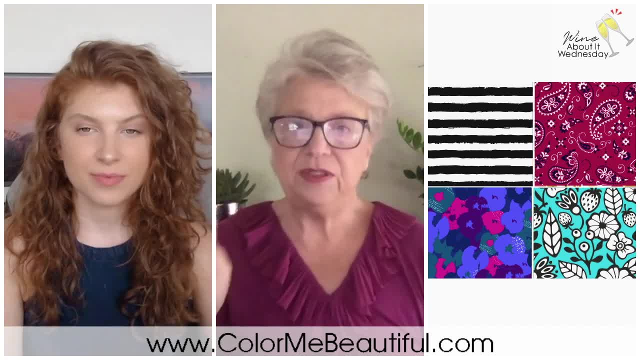 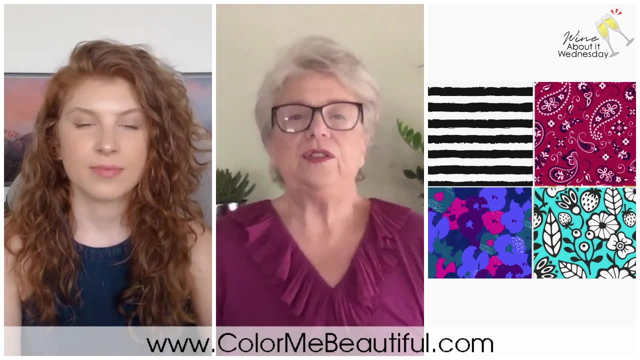 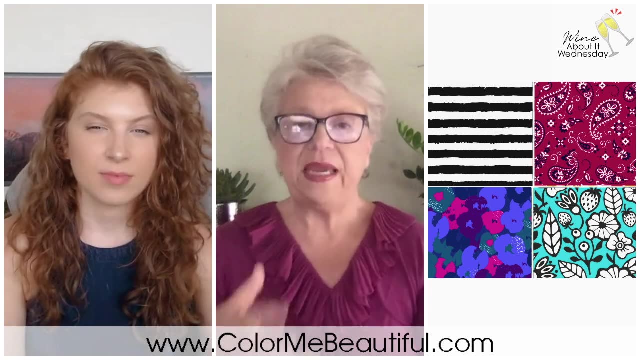 really bold contrast. and then in the patterns. the patterns are high contrast. be there and their heat color and light color and vivid color. and then on the lower left hand side, I wanted to do something that was strictly color and not doesn't have a lot of contrast with the fact that the colors are so different. 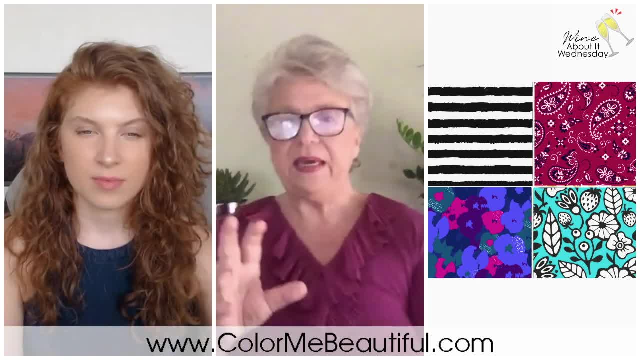 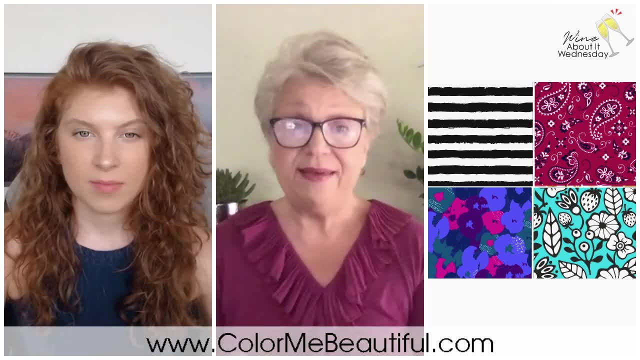 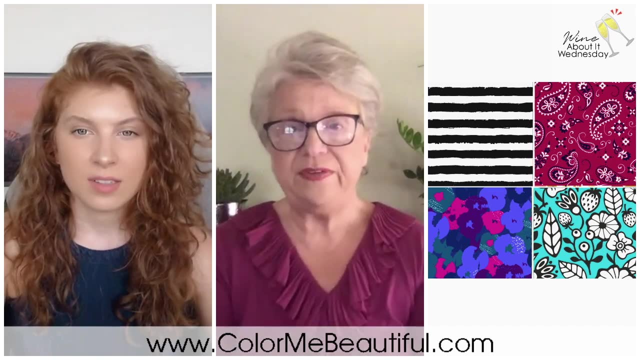 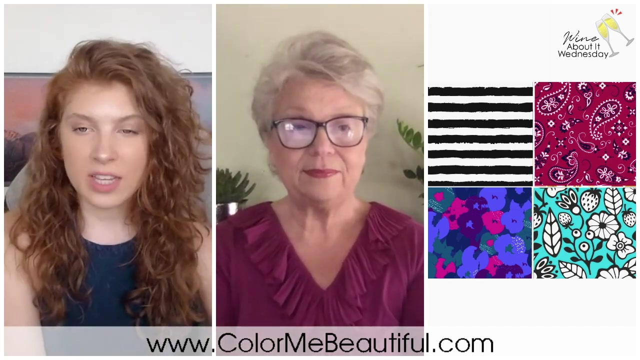 different than what that? um, there's like a hot pink color in there next to that beautiful contrast. I mean, technically it's not contrast what it is mm-hmm, because you know there's a lot of right, of course. I kind of a fun musical very high contrast combination. and another thing I was just thinking about is also: 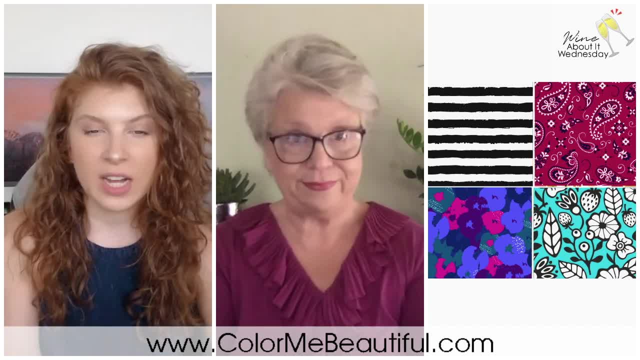 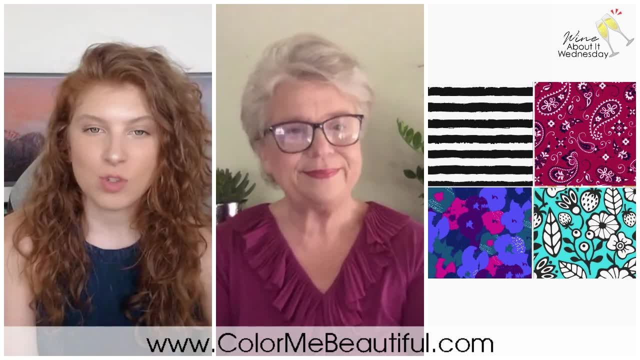 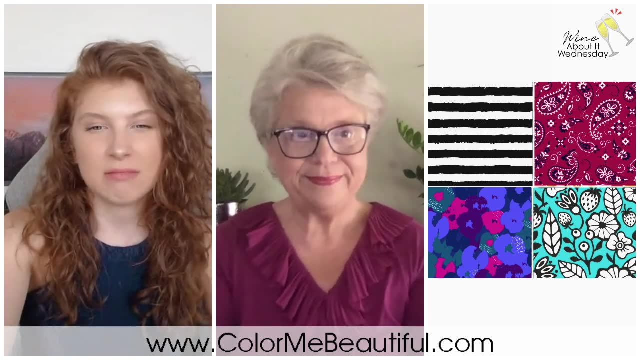 silver. so if there's silver in a pattern, you kind of get that a lot. when manufacturers kind of just try to spice it up a little, they always add some type of jewel tone. so silver, if you see silver in there, that's also a cool season. that's kind of like a tail, a telltale. yes, all right. so now that we've 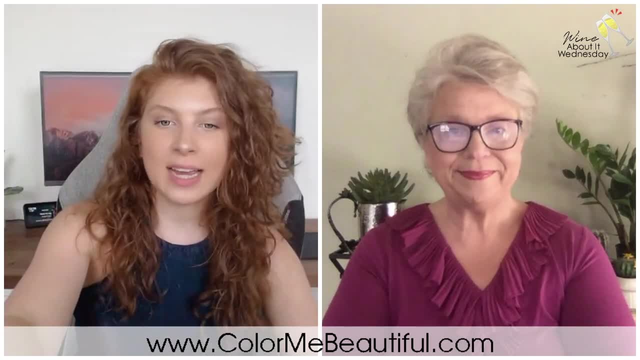 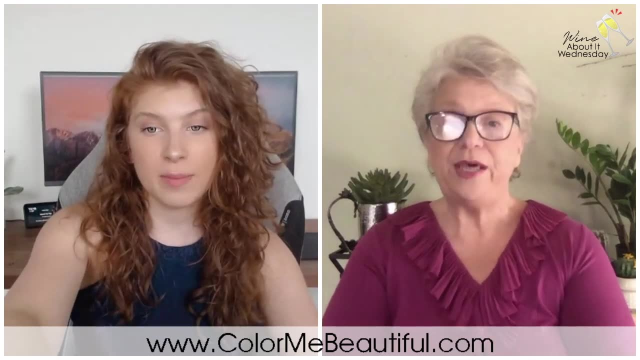 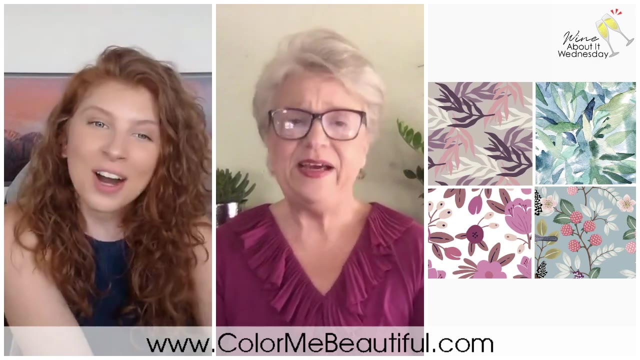 gone to winter, I'm gonna hop on over to summer so you can kind of see the difference between the winter and the summer, and but both of them are very cool. so let me know, the winter was high contrast, mm-hmm. now we go to low contrast. I don't want to say it that way because it sounded like we went from. 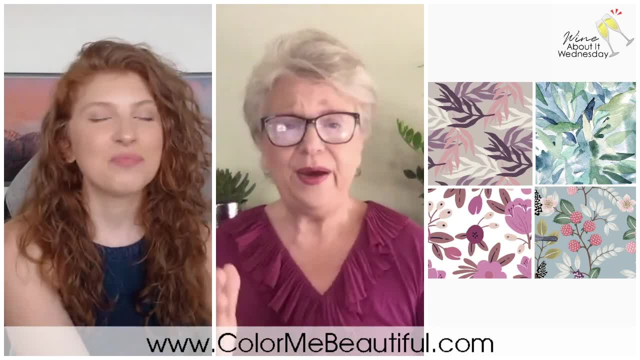 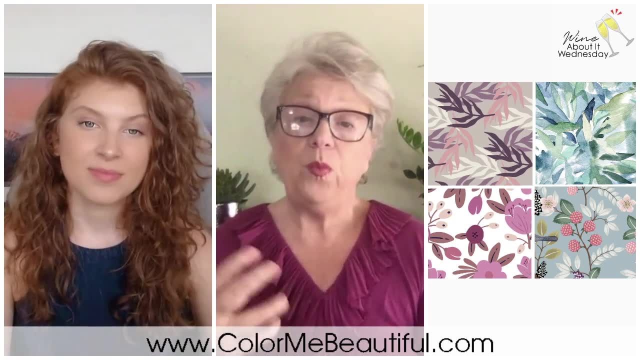 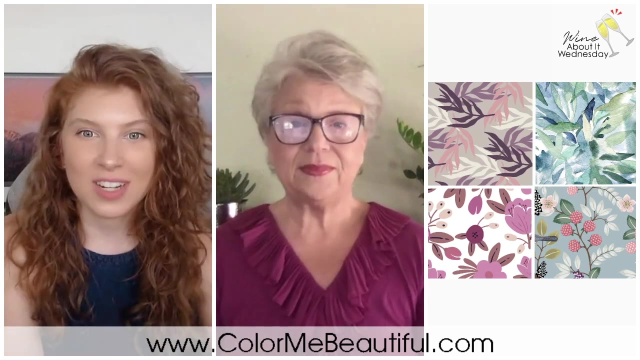 energy to no, no, no, no. there's a sophistication in the winter palette that I love: mm-hmm. and when we say low contrast, that's good, that's fine, it's beautiful. well, look how gorgeous these patterns are. I love all of these different patterns. we do, yeah, and the idea is you. 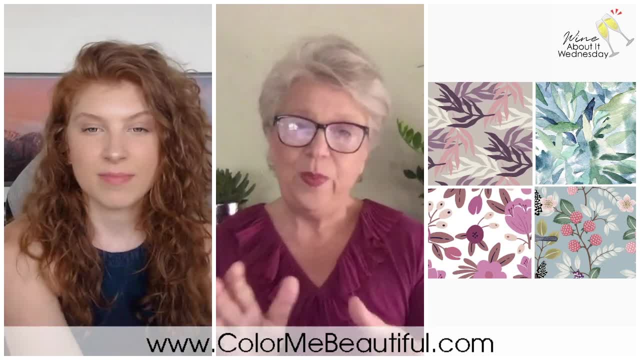 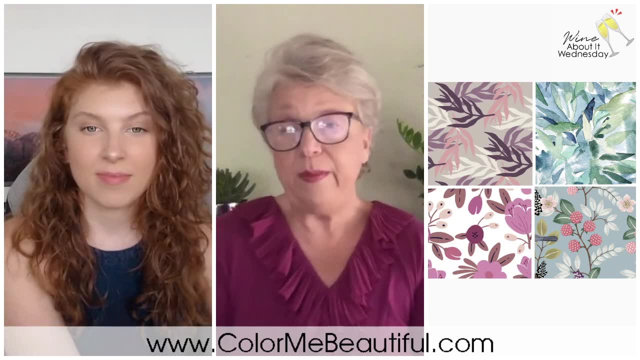 can wear any color if you're a winter, but you just want it to be a little bit more powdery. and all of these four ones that I would, that I put together for this, I would wear this in a mask and wear this in a blouse. correction, this is. 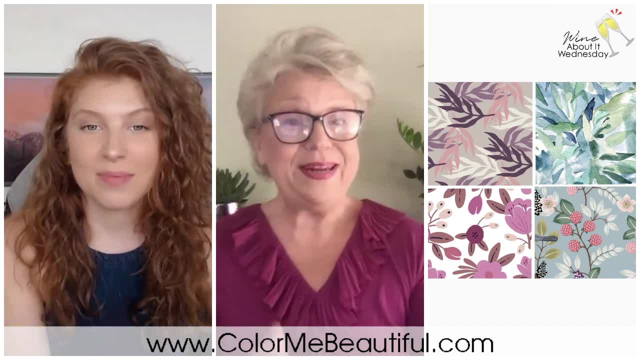 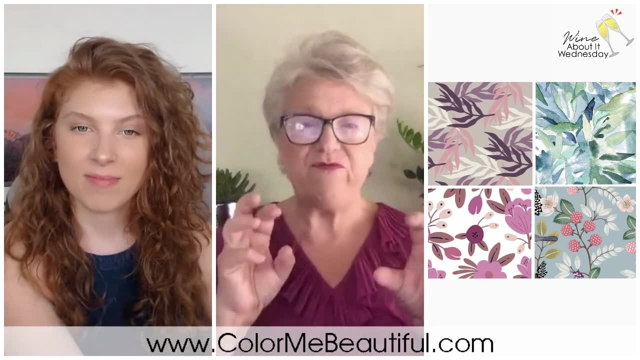 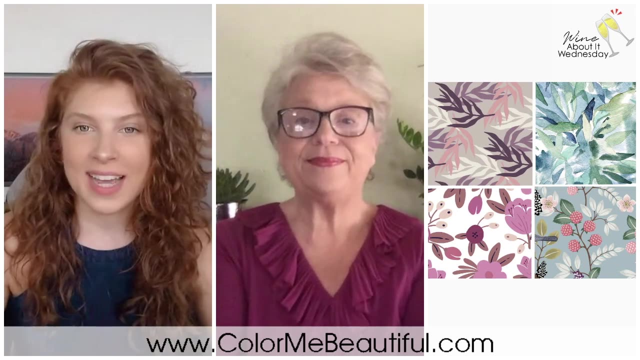 the summer palette. sorry, not the winter. this is. I'm sorry, did I say my hair accidentally? but it's okay, it is the summer palette and the end. what you don't see is that vivid contrast. yeah well, yes, it kind of just calms me down. it's very well. honestly, I love all of these. I think they're all. 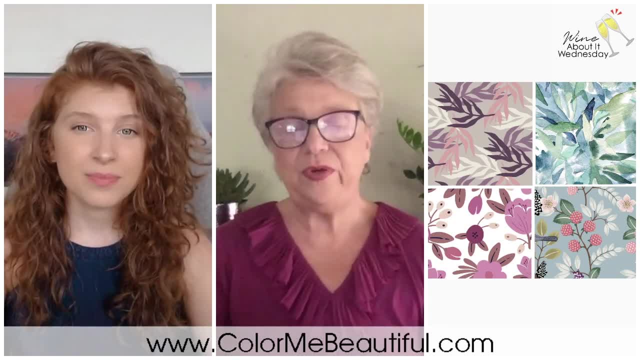 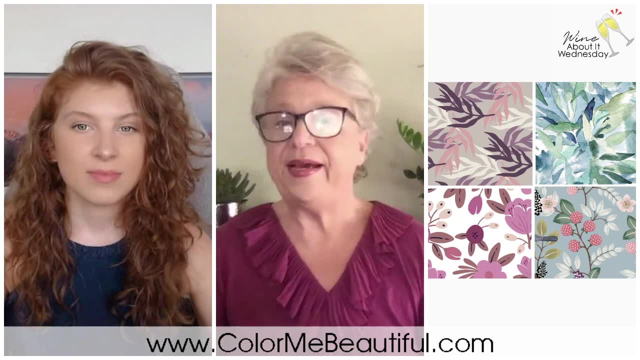 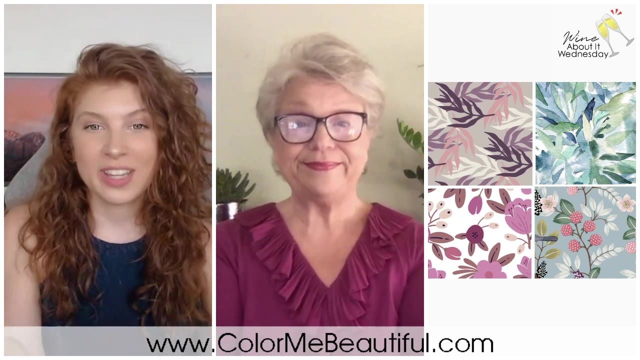 gorgeous, mm-hmm. and it makes it easy for you to kind of envision them on someone of my hair color, or someone with blacks and blonde hair. no red or gold highlights. um, what can I say? I could see you in all of these patterns too, like I love all of these. they all would look so good on you, for every. 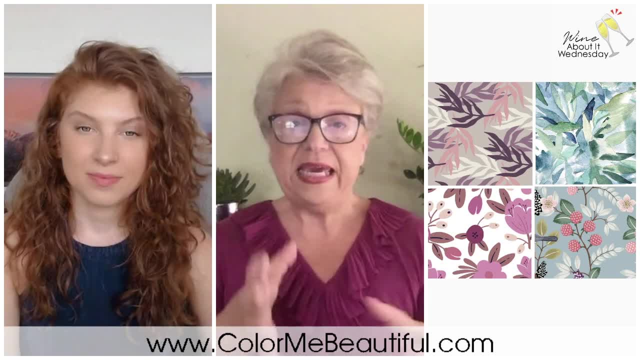 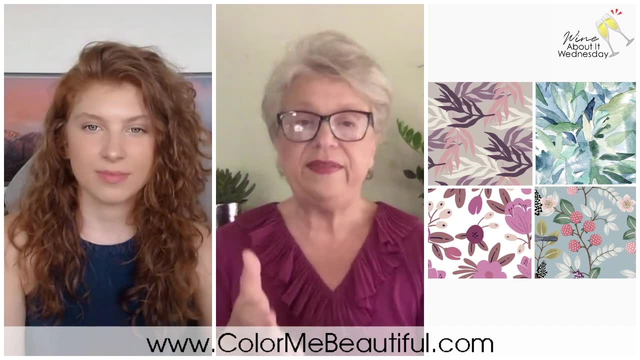 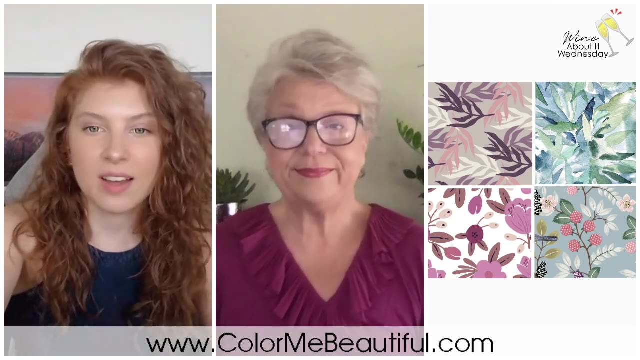 summer out there. so any of you summers out there think in terms of patterns that do not have a lot of contrast and, um, that are soft. that's your buzzword for summers. think soft, mm-hmm. I love this. these are gorgeous. I absolutely love these patterns. I kind of want them. can we turn them into autumn version? why? 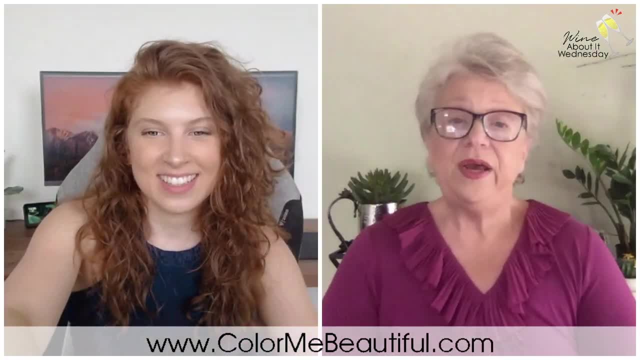 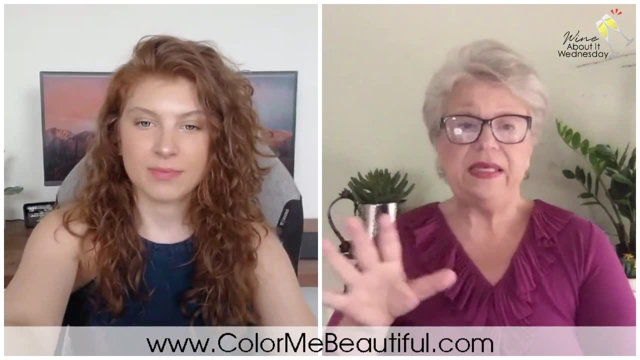 don't we look at the autumn versions and see what we have there? and you know I was. well, you want you, let's go back. oh yeah, I was gonna say now if I fell in love with the one in the upper right, any of these for you? I? 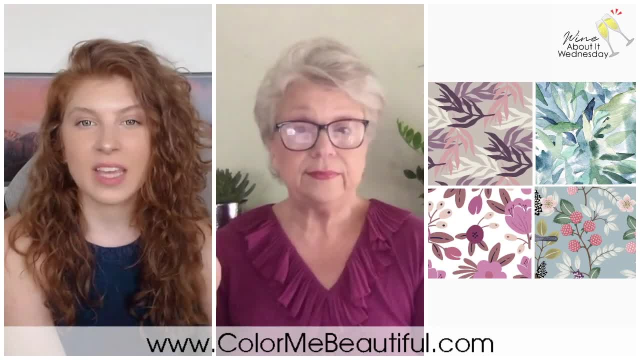 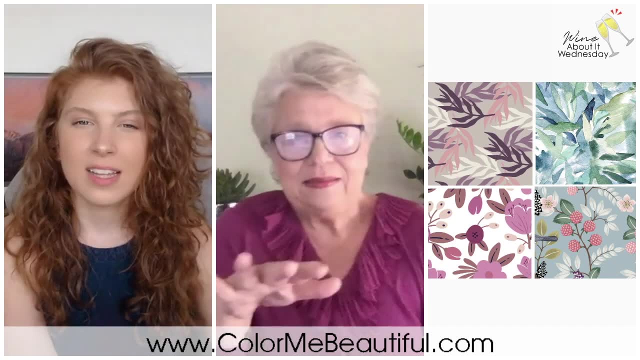 could, if that one you could wear, mm-hmm. yeah, the blue and green one, mm-hmm, so that one kind of bridges across the two warm seasons, because it, yeah it, but between the two soft seasons. I'm sorry, right, right, because it is soft, but you. 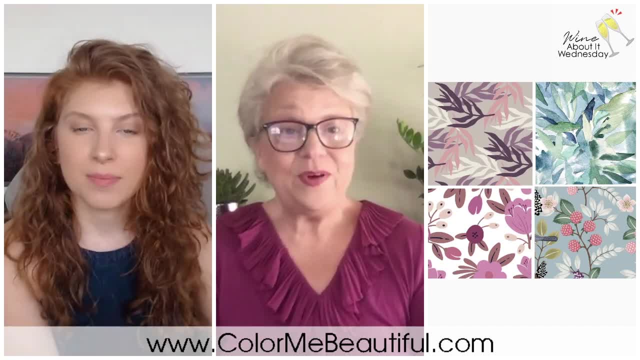 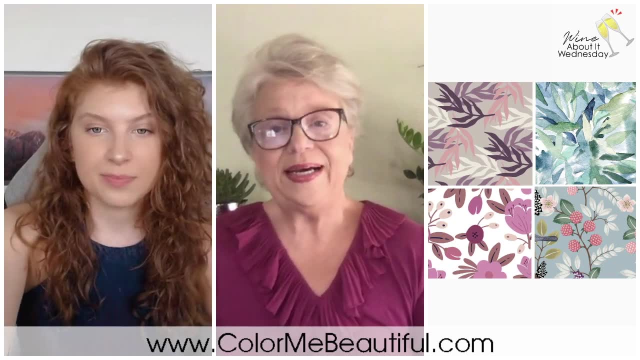 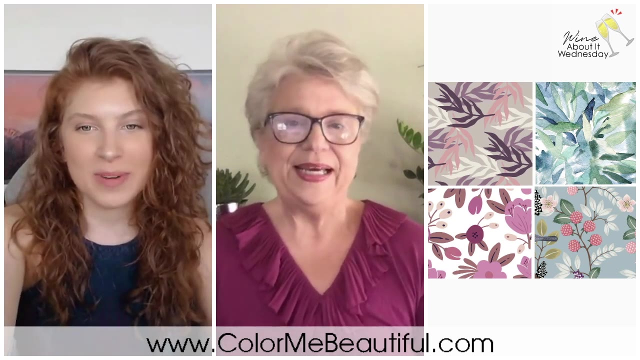 know it has some very neutral blues and greens going on there. you know what's crazy me? at the same color eyes and our eye color is picked up in that color, right, right watch. so yeah, you can have that one, but that's the only one. why can't I pull off that bottom right with the strawberries? 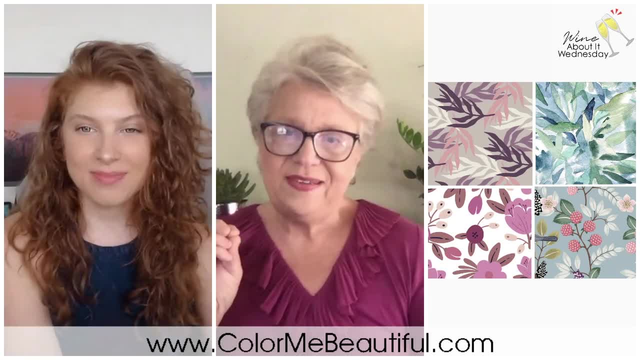 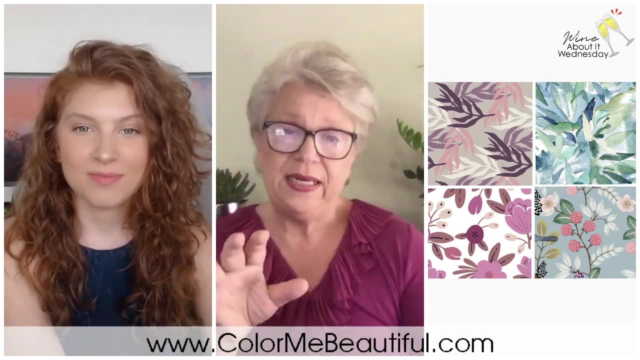 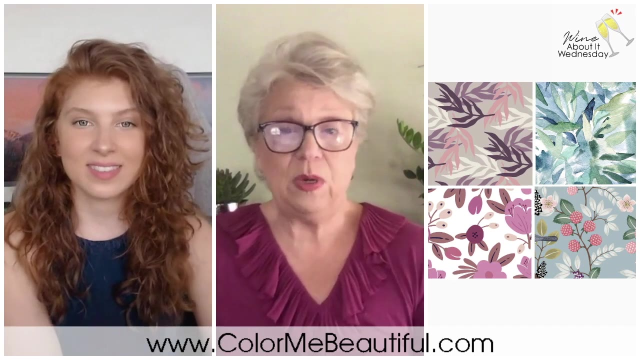 those are so cute because I think you need just a little more work. it is the berry, is watermelon, and everybody can kind of wear watermelon, mm-hmm. but I think I would like to see more work and I'll make a switch for you. well, you know, I did your trick where I 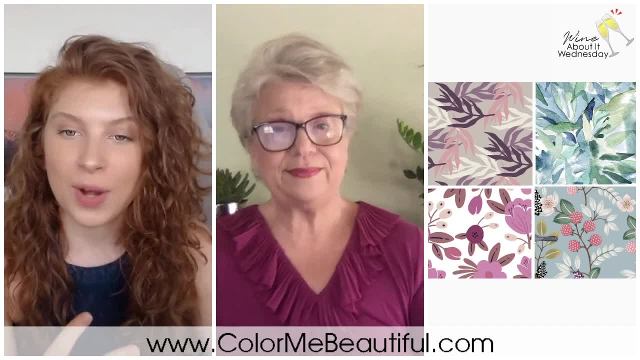 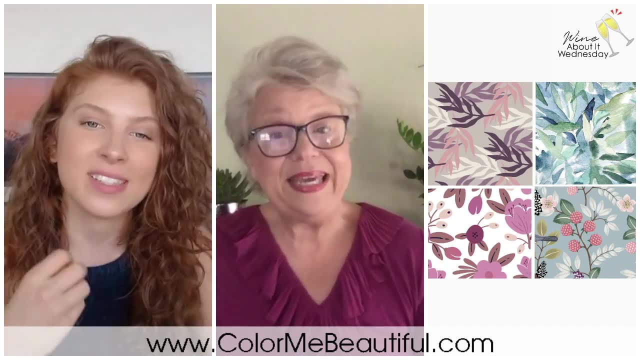 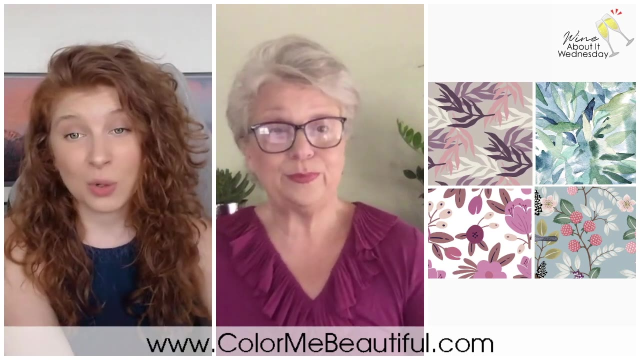 blurred my eyes and I tried to see what that in the bottom right, the color that really shows out, and it's that soft, pale blue which really just makes out of summer, and it leads toward gray, which is that on your right, right. so it's absolutely gorgeous print, but it's definitely very, very cool everything. 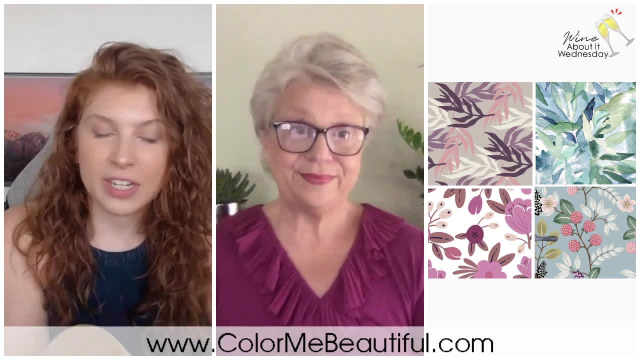 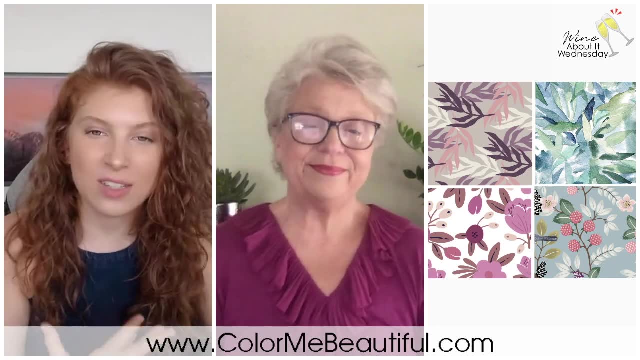 about it, and when I do that kind of trick, the blur blurring your vision trick, I mean all of these, like I have that background coming through, with the pinks also showing those pastels- soft colors though- that I have a funny story about work and the blurring of the eyes, because this is 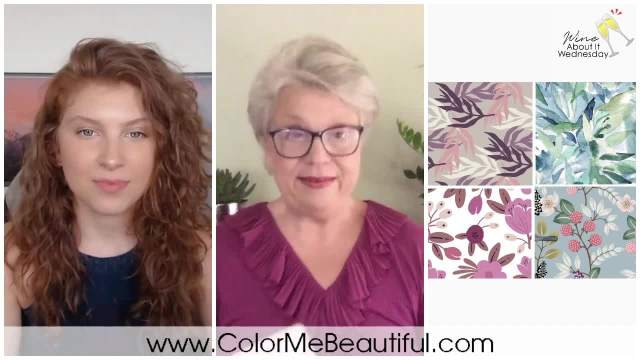 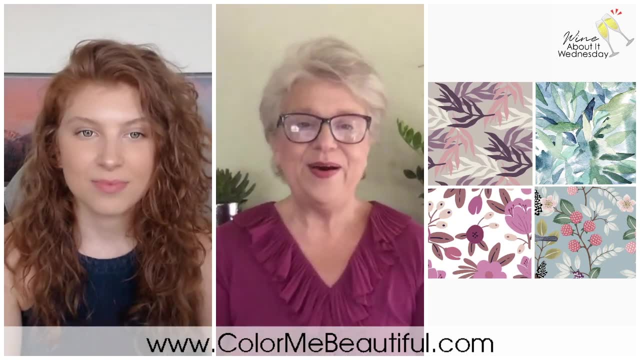 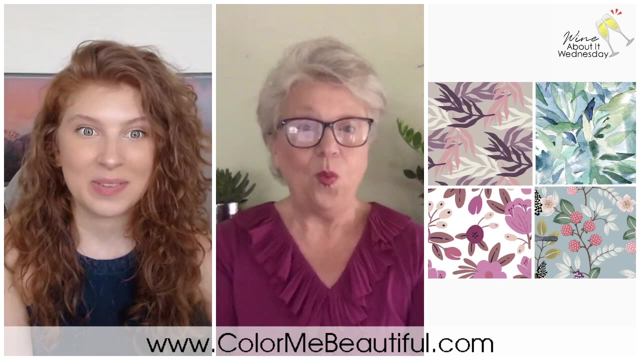 my job. I do this all day long, and, Sarah, you do the same thing, but I am a big fan of the blurry eye trick as I'm posing and creating, and so I think, at least twice a week, the CEO of the company walks in the office and what does he say? what's wrong with your eyes? you know what's wrong. 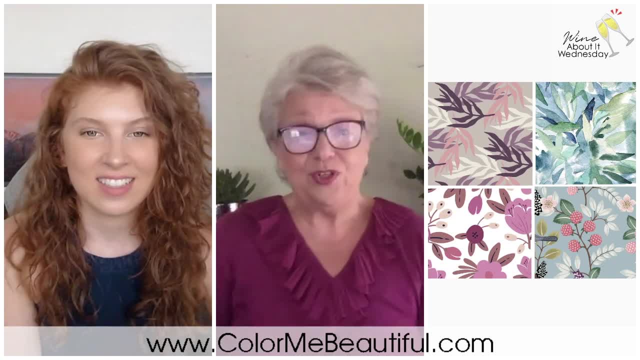 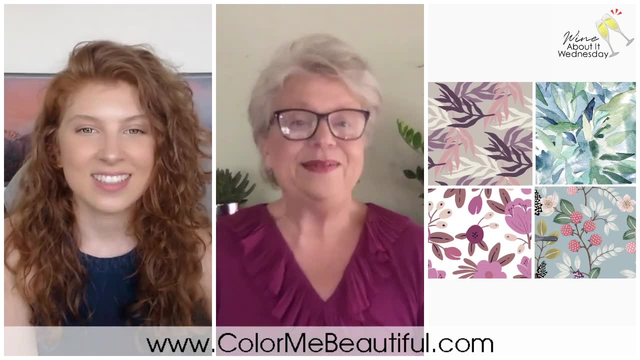 with your eye, and I've been doing this at that company for 20 years with the one eye closed. yeah, yeah, he says: do you have a problem with your eye? is there something going on? uh-huh, that's just what we do. yeah, you definitely have that. 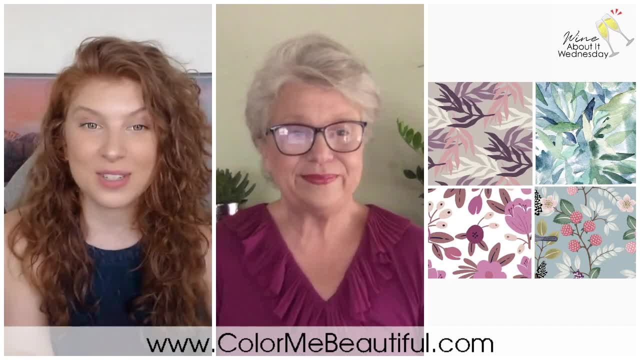 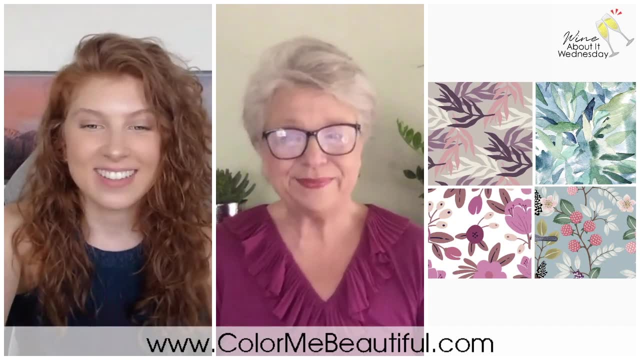 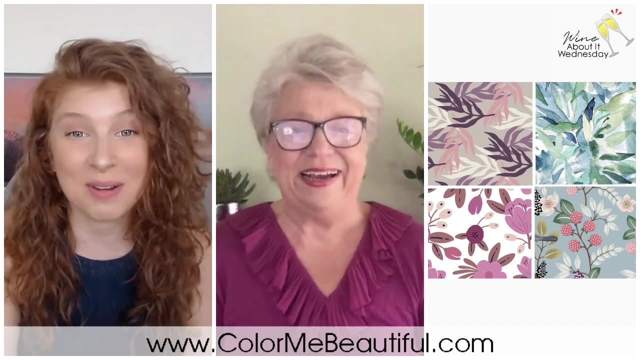 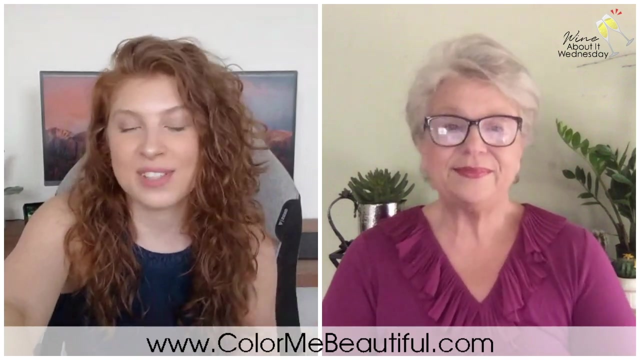 artist thing where you always close one eye and your other one starts twitching when things get serious. when you close one eye and your other ones start switching, that's when you know the serious color business is going on all right. so we were just talking about being soft, all those soft colors, and 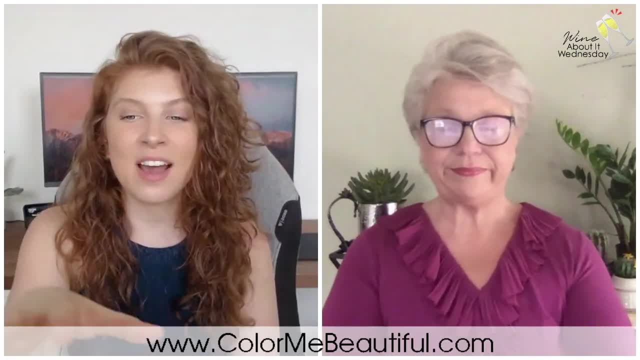 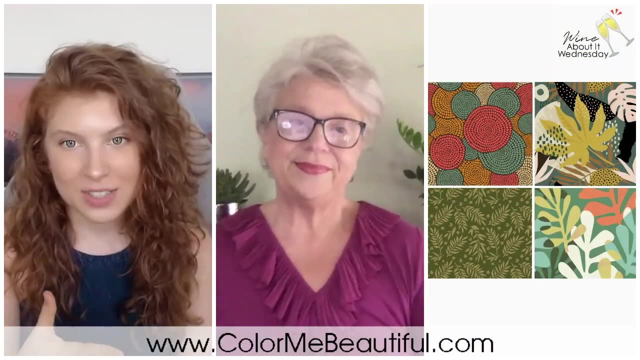 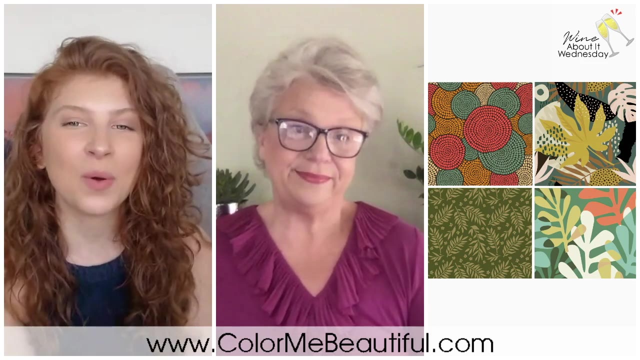 that's cool. we've dealt with both the cool season, mm-hmm. so now I'm gonna stick with the soft, but we're gonna switch over to warm. so this is gonna be our autumn colors. right here you can wear these, all of these greens, i love. i love these warm, like terracotta, corally kind of. oh, they're all so gorgeous, i love. 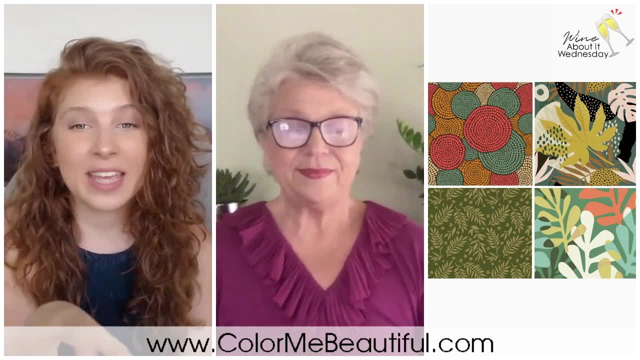 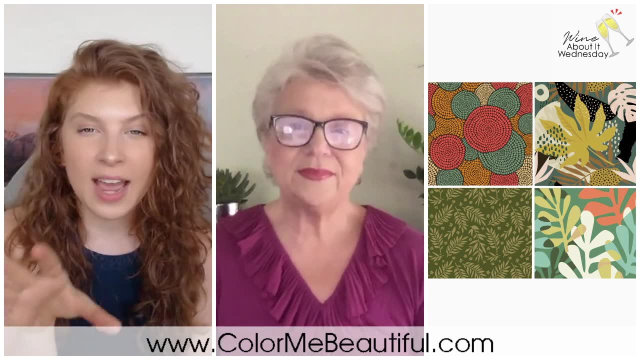 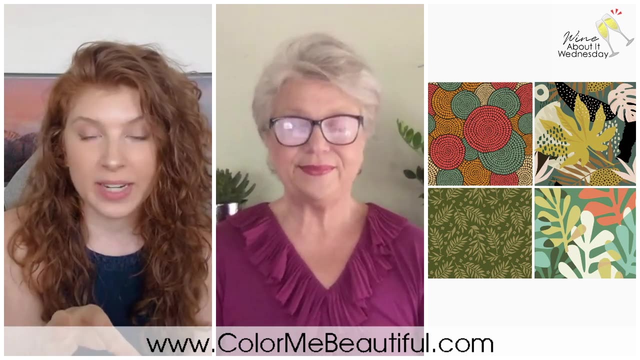 them. so now i i'm picking up a lot of greens and all of these. that's kind of like the overall theme i see, and when i do go a little blurry i notice the oranges and the corals in the top left. so i'm really getting that from that print. but if i move over to the right, that one leaf in that middle. 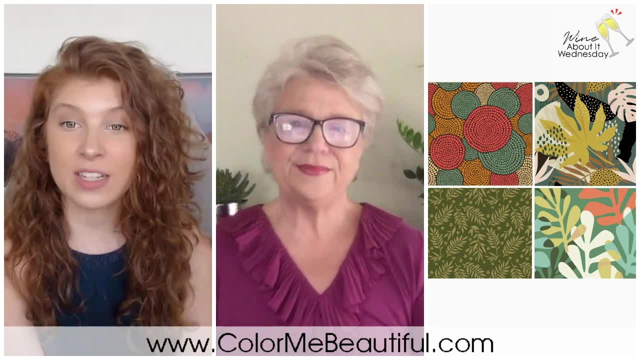 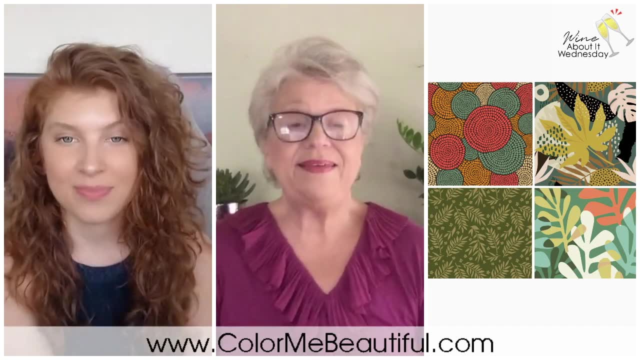 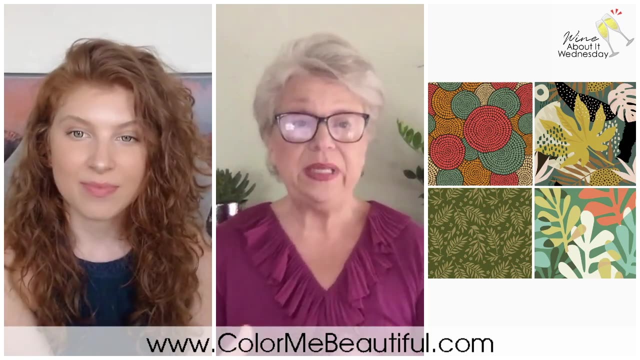 that soft green that's a little bit lighter. that's what's really showing through. but i noticed that there's also some black and white in the pattern. well, i did that on purpose because even though you're a soft season in your patterns, if you notice you can actually wear a little bit like. 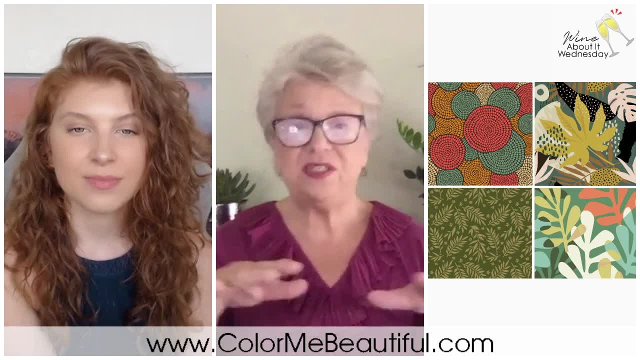 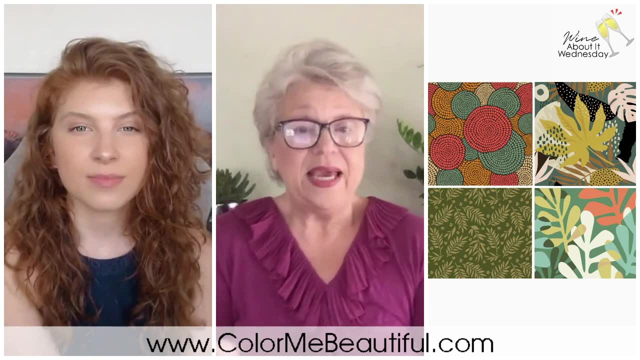 if you looked at mine on a soft season, there was no depth, it was just soft kind of across the board. if you have more depth of color, that means you can have more depth in your patterns. i wanted to make sure that i illustrated something that shows kind of a foreground. 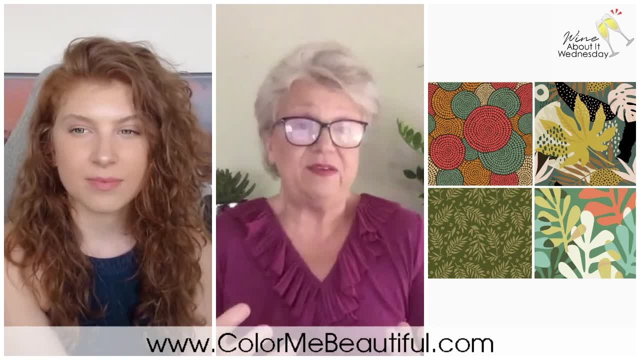 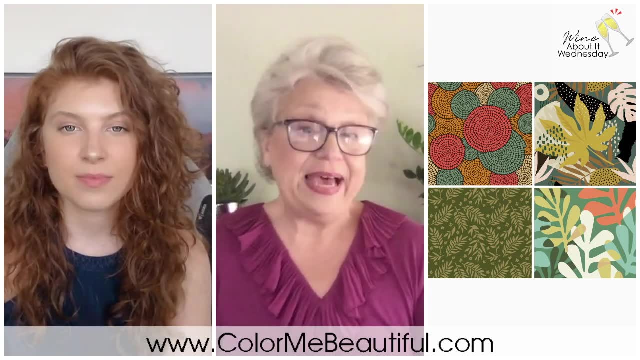 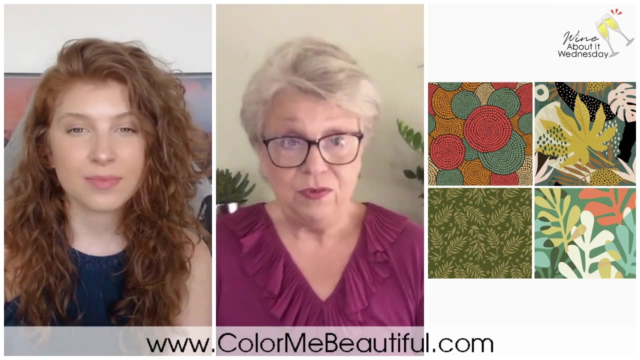 and a background, because if you're coloring, the fact that you've got so much of it, um, you get a little more depth, you're allowed a little more depth. for example, the lower left, that pattern, it's almost not a pattern, it's a color right. so in a color that's beautiful on you. 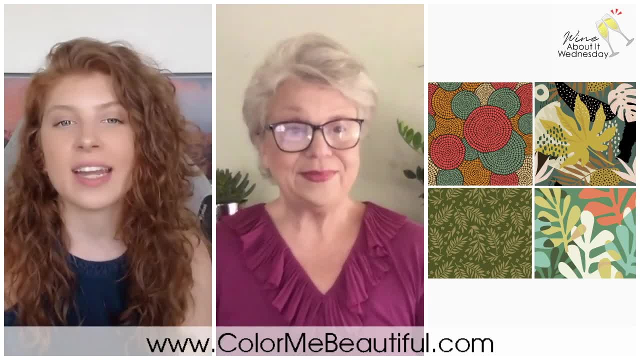 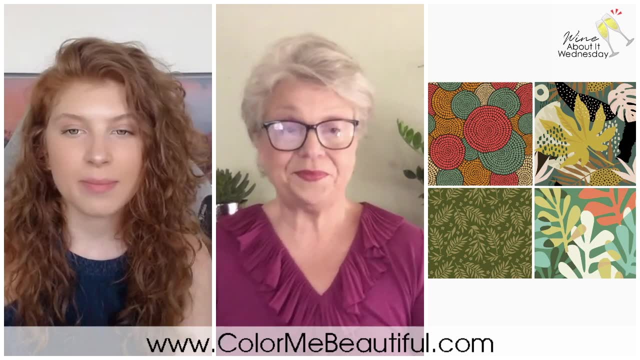 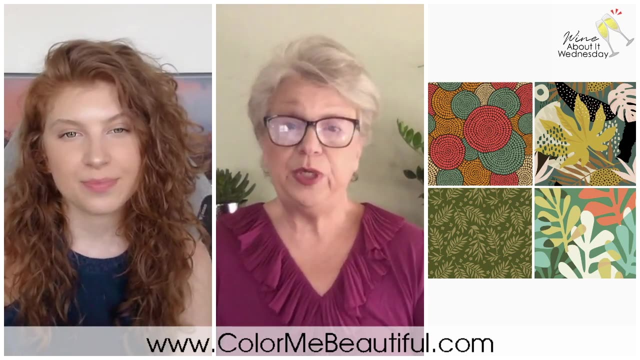 don't get me wrong, but, um, it doesn't have a variety. it doesn't have that variety that the others do. it that's okay, yeah, now, um, what about if a print has other colors that are in a different palette? uh, the, uh, the flurry eye trick is the trick. um, and i, i deliberately didn't choose. 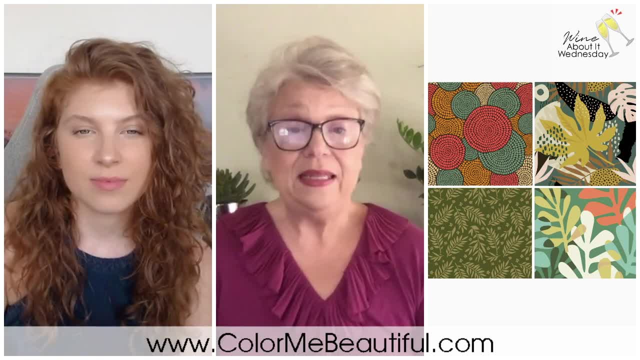 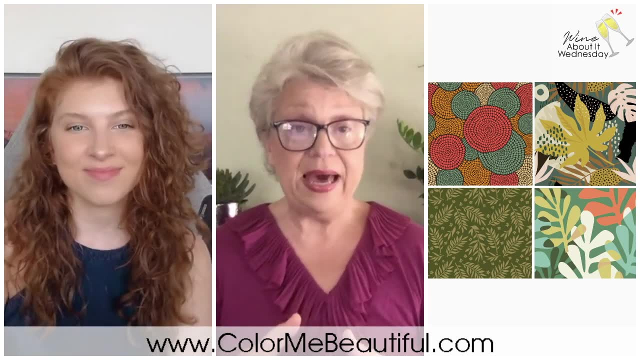 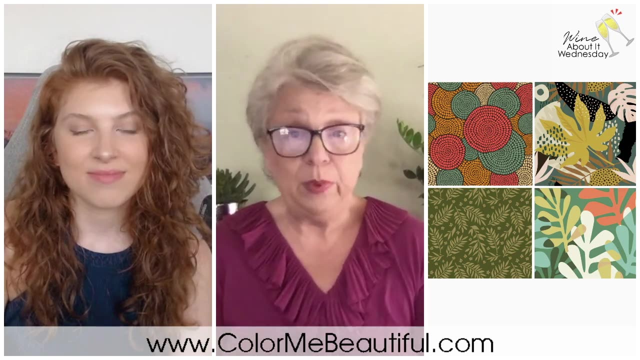 um, prints that had a variety, and you know what. they're hard to find because once you become attuned to this, you are not likely to find patterns that have a bunch of various in them, because things- even fabric designers- want something to be harmonious. let me give. 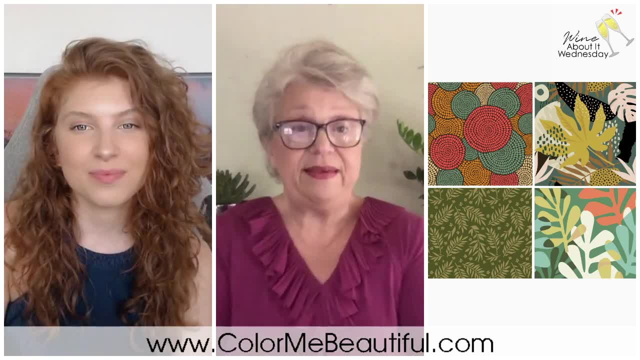 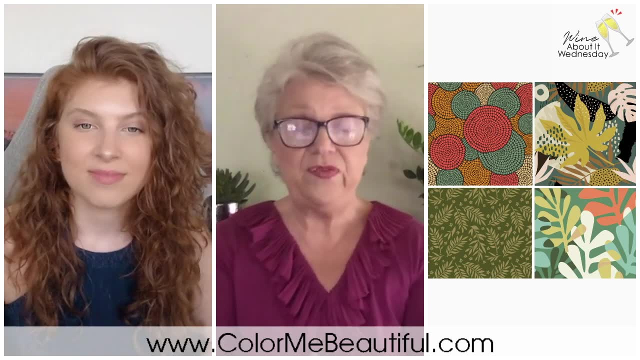 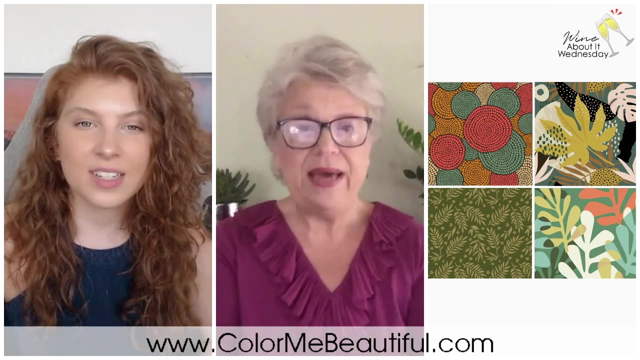 you a great example. um, leopard is a great example. you'll see all sorts of leopard in all sorts of colors, but inevitably they tend to live in their own color family and you don't see a lot of that. yeah, they kind of, but if you do, uh, if you do, it's like um a great. 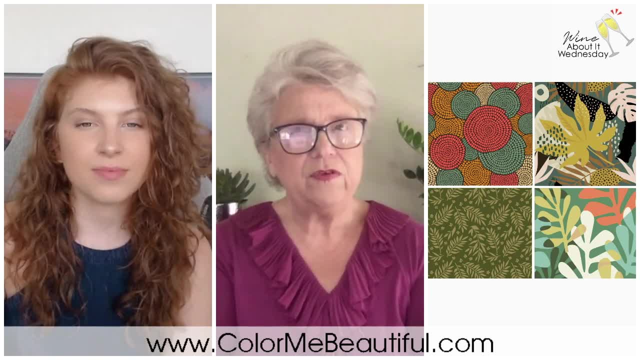 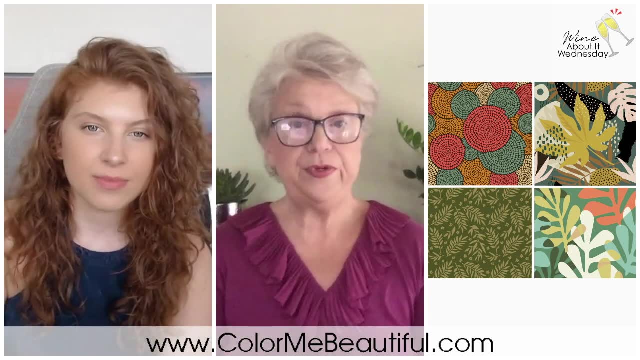 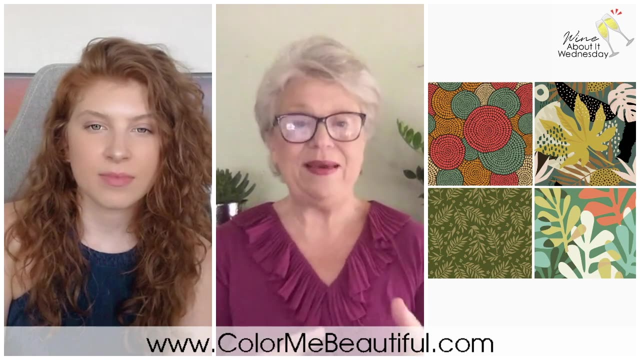 example is burberry, right? yeah, so we're. if you go on the burberry website and you look at their scarves, you know they're two thousand dollar scarves, so you know somebody has put some time into the colorway to these scarves. it's a perfect example because they are all seasonally appropriate. 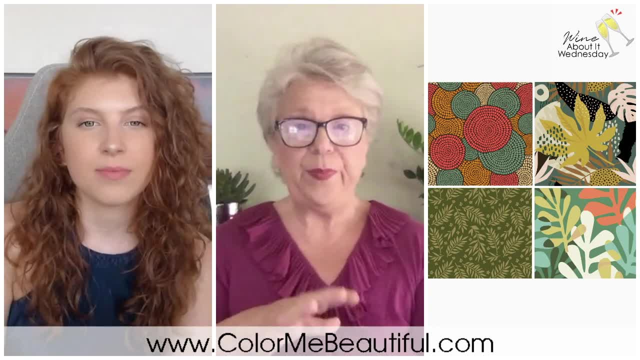 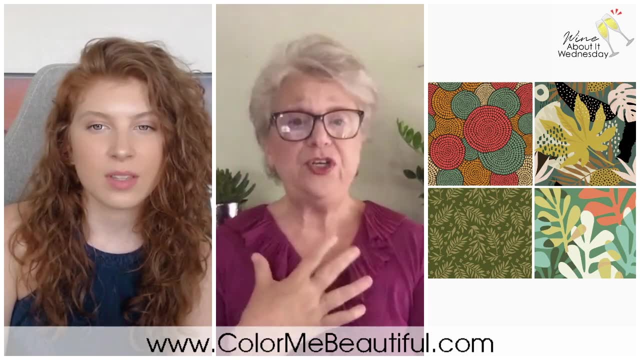 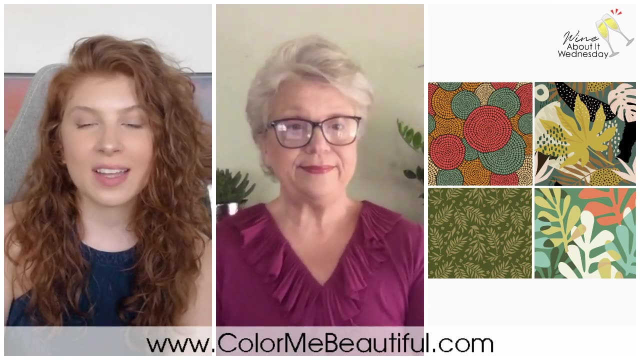 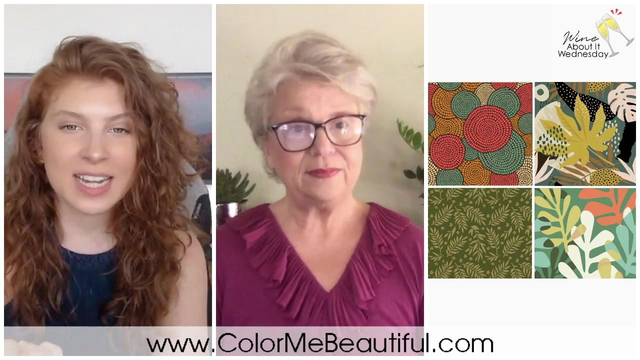 and rarely would you see, uh, a palette like any of these, um, that i have here for autumn, with a magenta- or just imagine my shirt color- thrown into any of these. what would happen? yeah, well, i i immediately think those soft colors that we just saw, um, like that soft blue kind of thrown in, would stand out. 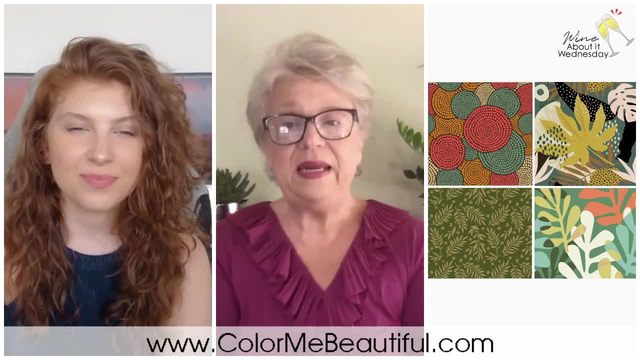 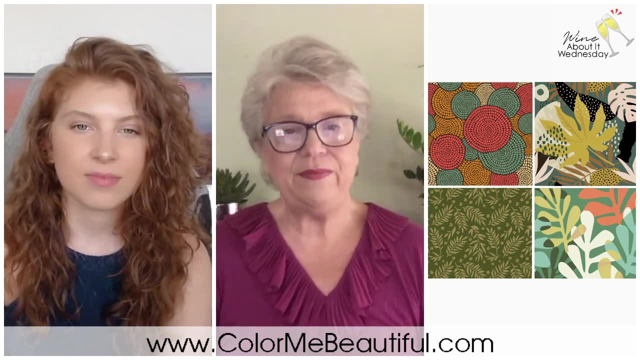 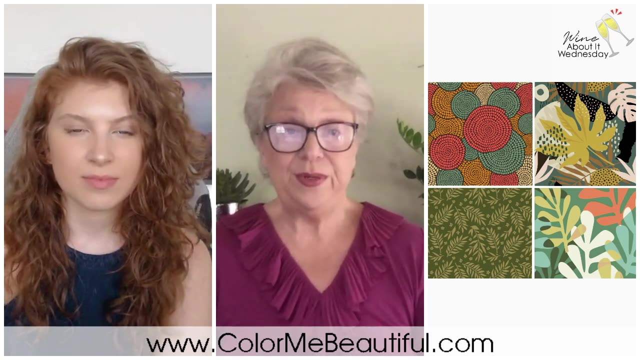 like a sore thumb. you know they do and and it's kind of like, it's almost like for the most part, and- and i'm talking about high-end clothes here- i mean you could, you can find some well-in patterns when, when the people who are designing the patterns know what they're doing. 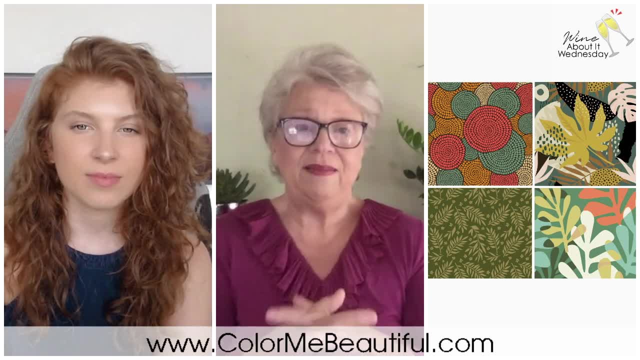 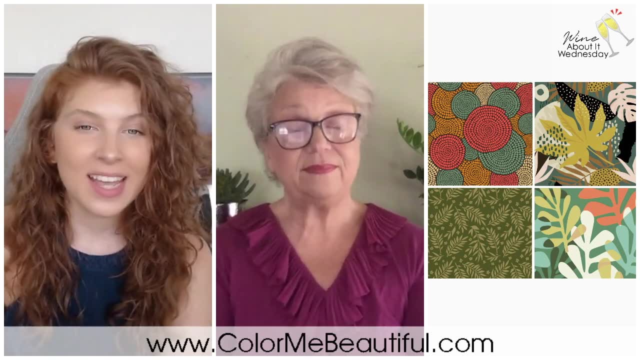 you. you tend to see them of a piece in in the same color and all of those colors harmonizing together, because, at the end of the day, that's the goal. you want that harmony and you want it to be able to work with everything you've got naturally. so i don't know that i answered your question. 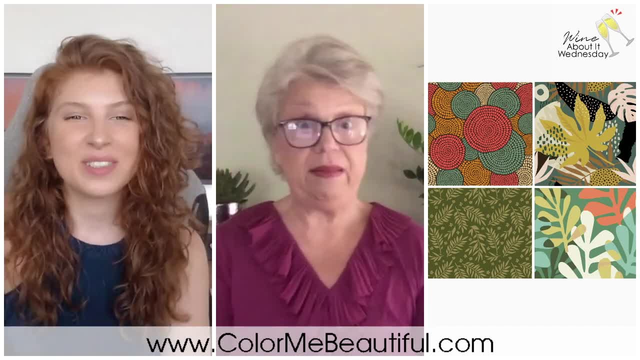 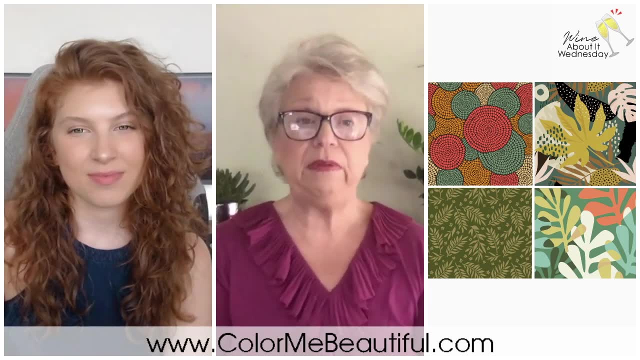 appropriately, because i got off on a tangent about my feelings about people designing fabrics and cutting them and being the right clip. but what i will tell you is, if you see a pattern that you've absolutely loved and it's all over the place, it's got colors from every season and it's just 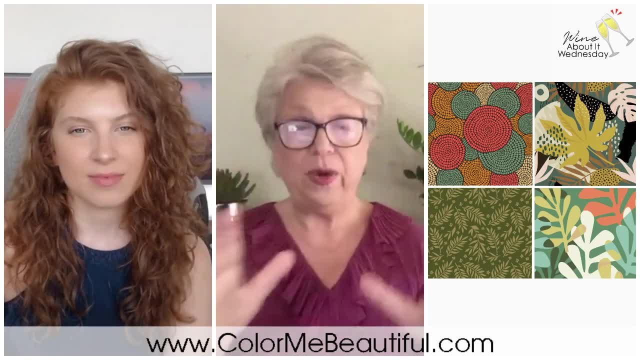 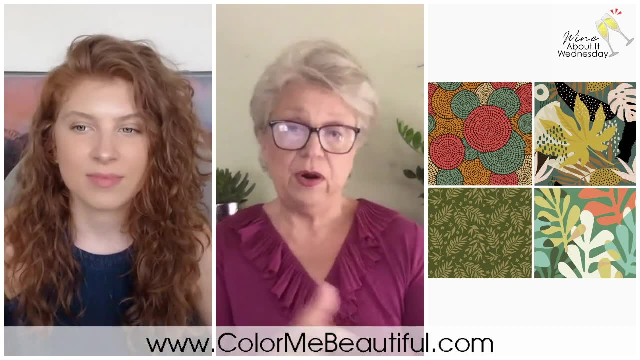 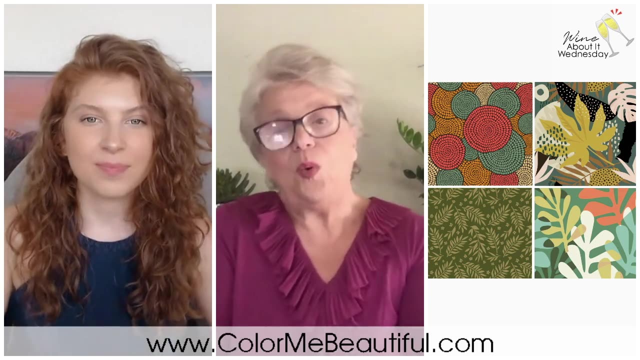 a hodgepodge and you know it's a jackson pollock painting, whatever. um, the thing is to make sure that you find a predominant color in that pattern that either flatters your hair or flatters your eye color, and then inevitably, you likely won't make a mistake, or go find a pattern that has 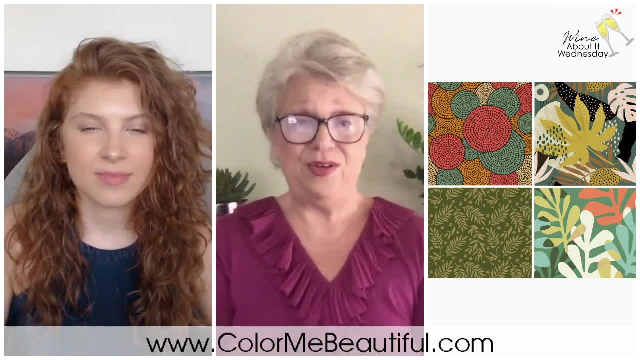 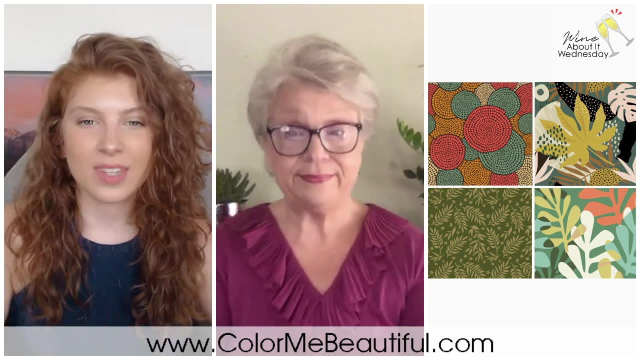 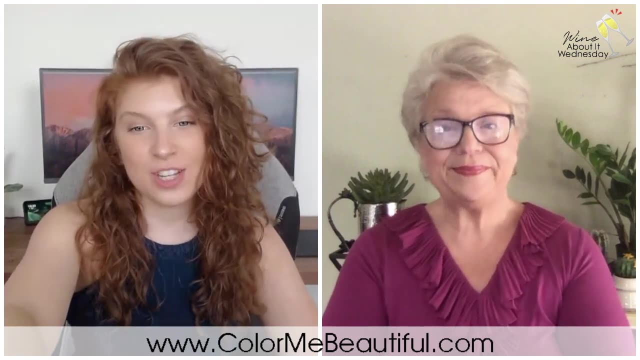 the colors from your ideal or your cup color band before you get short color. let's face it: at the end of the day, that's what's going to make the difference. all right, so done with autumns and our last season is going to be the springs, which 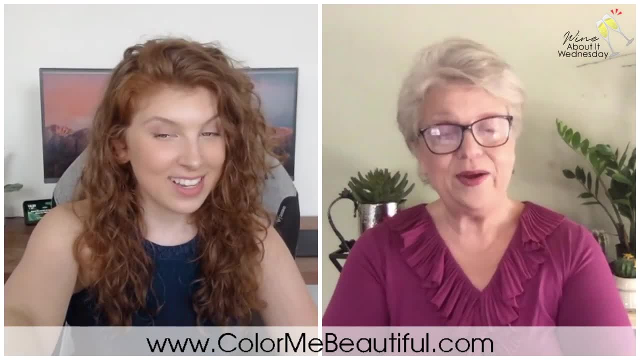 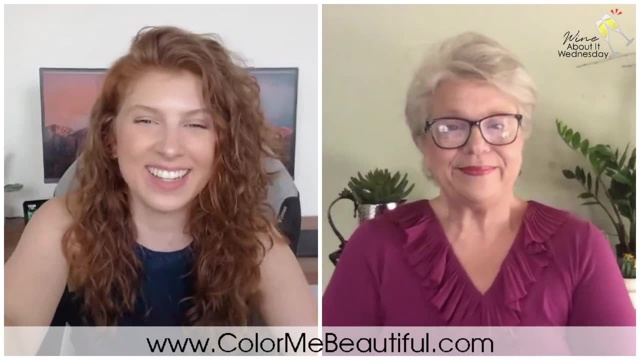 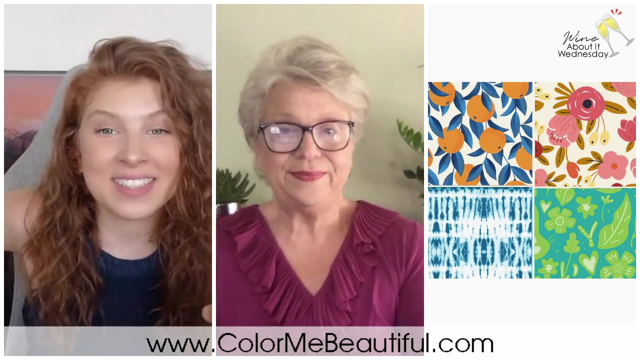 are high color and bright. they're high contrast and warm, right, yeah, you guys know it's warm, it's bright. all right, here we go once again, right there: warm and bright, boom, and these are. so i really like to see these patterns. this is the spring palette, but i really tend to see these patterns. 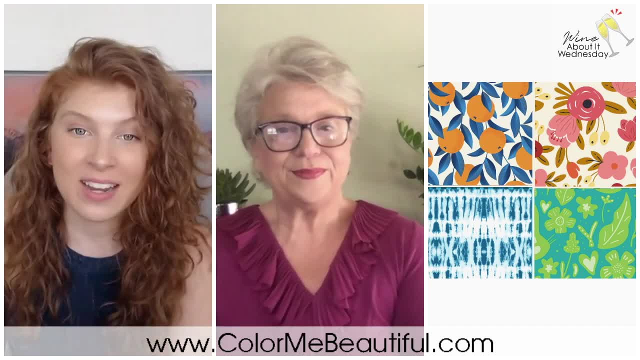 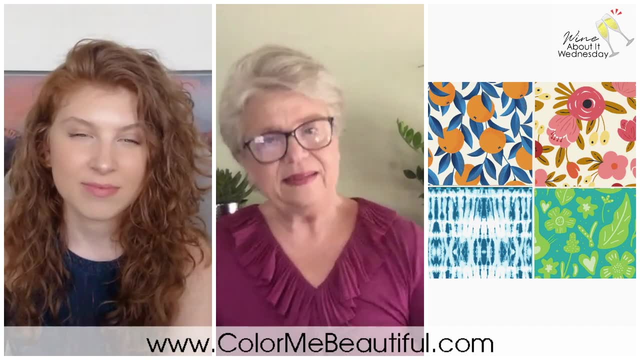 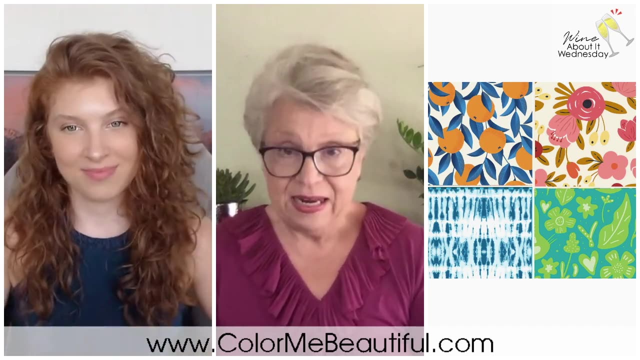 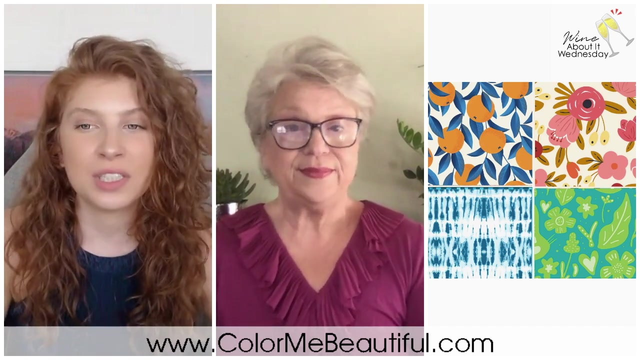 spring and summertime. so right now i am this palette right here. i see everywhere, uh, yeah, maybe, um it and yeah, like, for example, lower right hand corner, that green is a spring green. nobody wears that color better than a spring. that's what i'm on and it looks so. 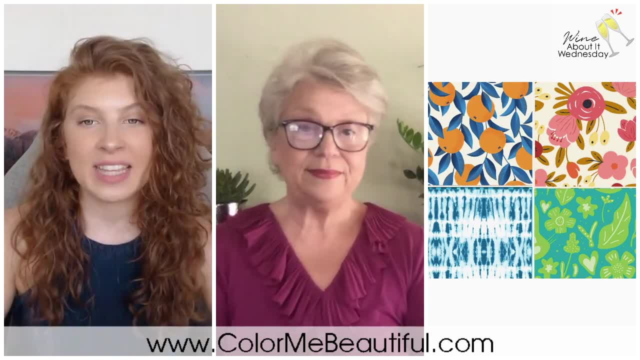 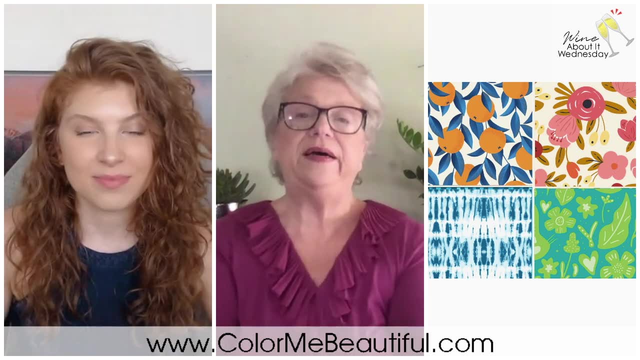 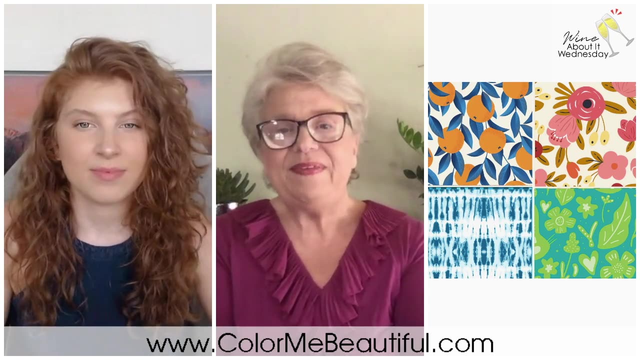 much like a spring if you're debating, if you're a spring and you can wear kind of like that yellow green- oh, it's such a good color on you and only splinters can wear it. now in the upper left hand corner. this one's kind of fun, because i thought about doing this with lemon, but the lemons look. 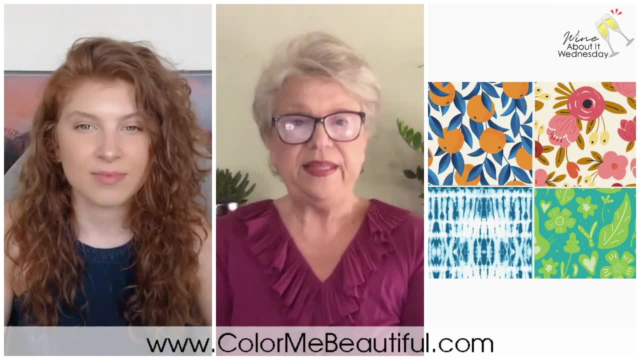 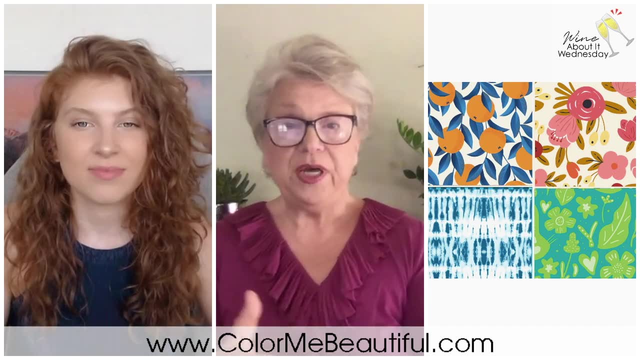 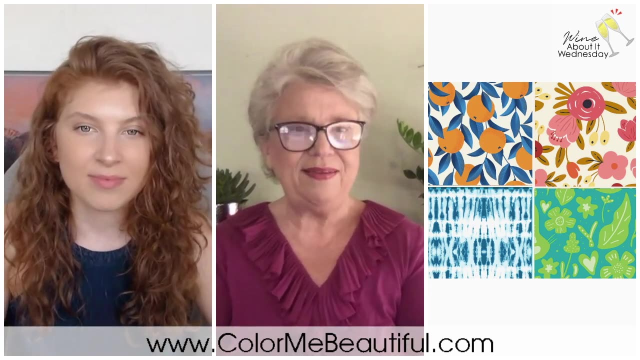 kind of silly on the blue, because this is, um, this is a complementary color scheme. remember last time we talked about complementary color schemes and how, um, if you look at all the different, uh, like colleges that their colors are complementary color schemes. auburn, this is alabama, clemson. 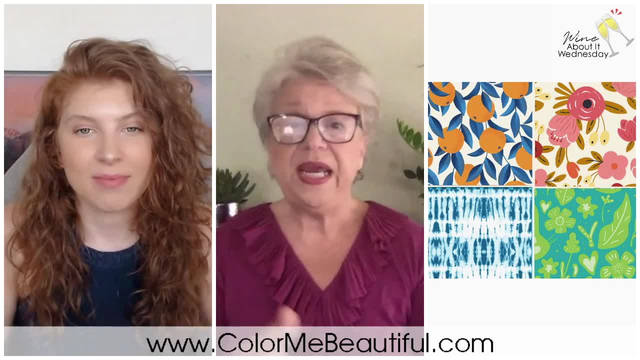 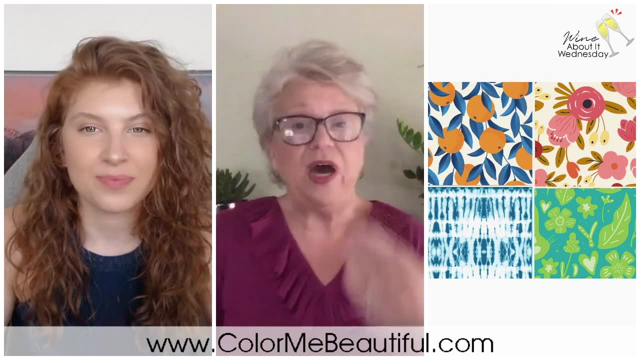 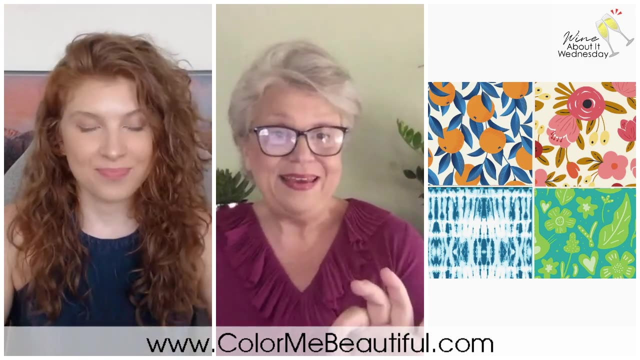 i don't know, i don't know that stuff, but um red and green, blue and orange, purple and yellow complementary color scheme. so i was thinking it could be done very easily to put the lemons in there and then if, if it was a lemony kind of an acidic yellow, winters could wear it. yeah, that. 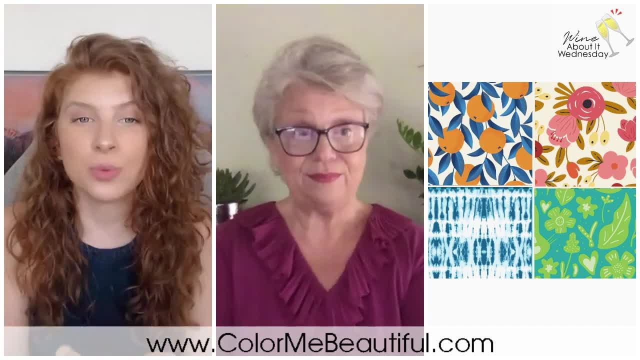 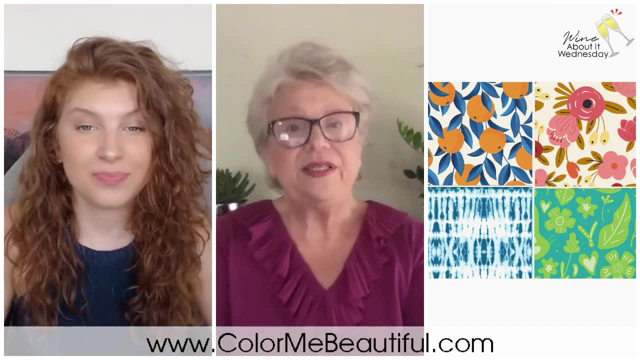 would be a beautiful print on a winter if it was a winter print on a winter print. on a winter print. the actual lemon yellow, not a golden yellow, but acidic. yeah, that would be gorgeous on the winter. so then i thought maybe i could do that for the winter. but i 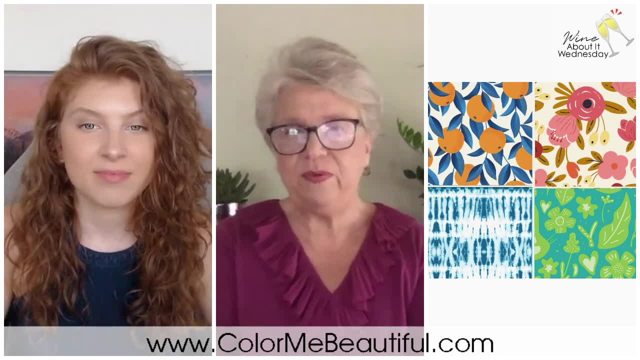 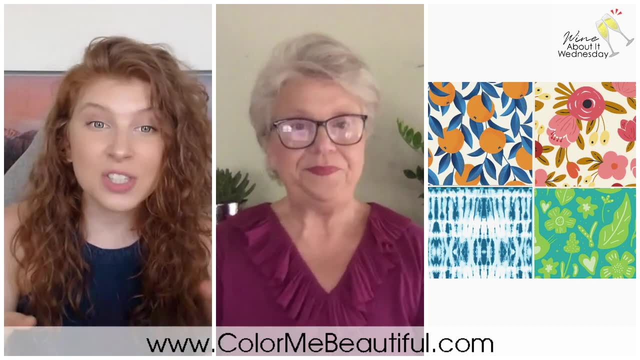 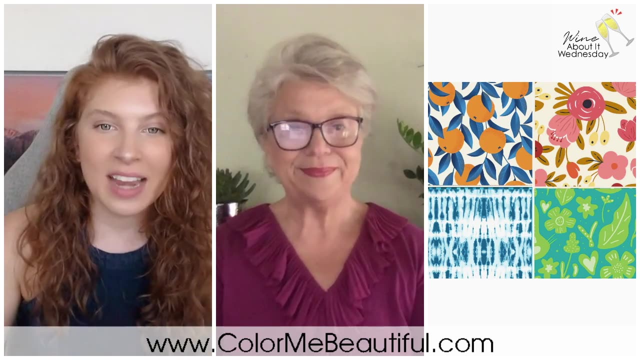 didn't want to because i thought this was so much better for spring. it does look. i really love that pattern. honestly, it's gorgeous. i really love that and it's so just talking about how one slight little change could move that entire pattern to a different season. so it's kind of mind-blowing how 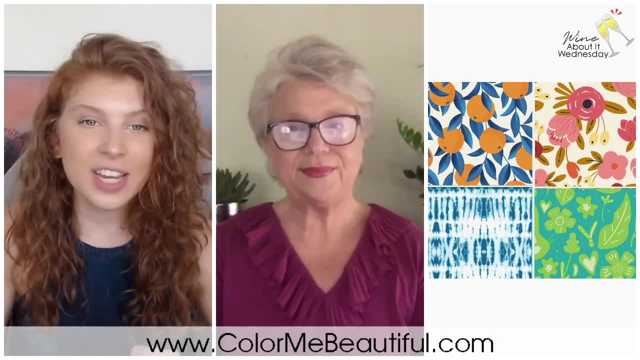 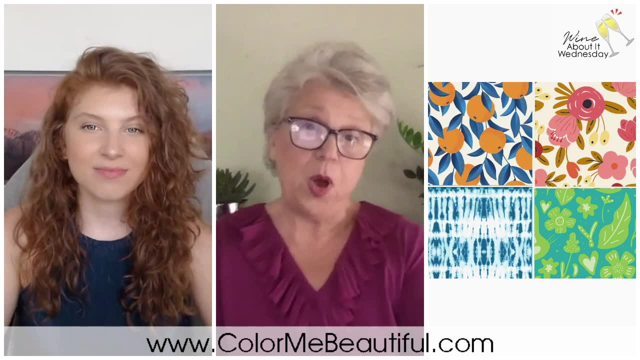 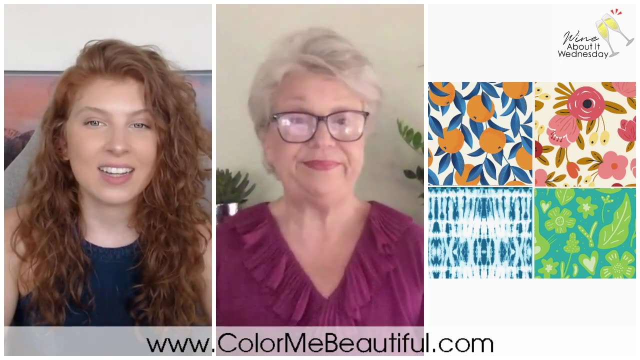 you know, just one little tweak or one little color change and that whole pattern would shift to a different season. well, the upper right hand corner is a perfect example. if the background color went from off-white to a pure white and maybe shifted a little toward what i'm wearing- uh-huh, i think. 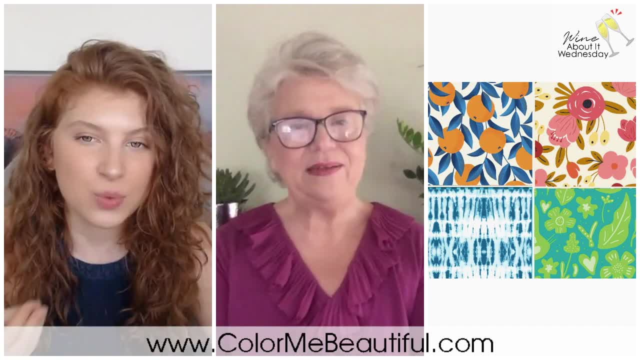 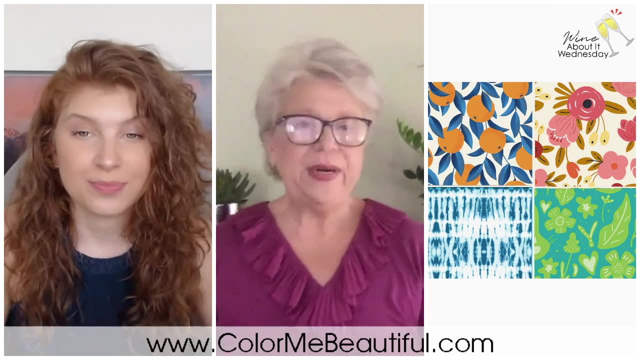 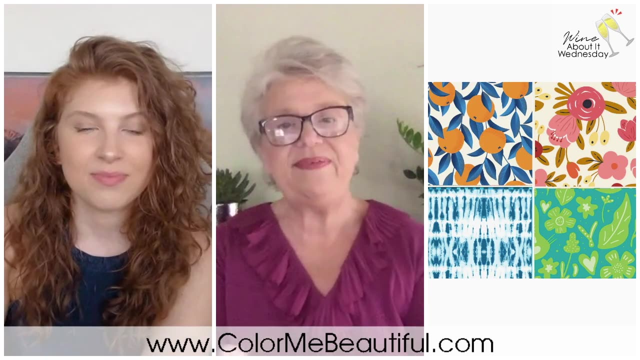 yeah, i think those leaves that are on that, that orange leaf, might be a little more uh-huh, maybe go um like a gray or something along those lines. that would be gorgeous on a summer. so, as you can see, it's not really the pattern per se, it's the the contrast within. oh, and this is the bottom left. 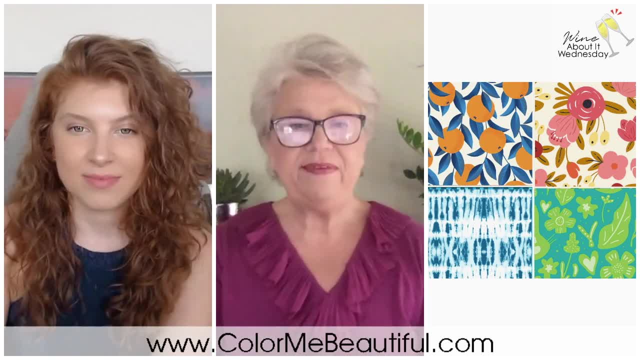 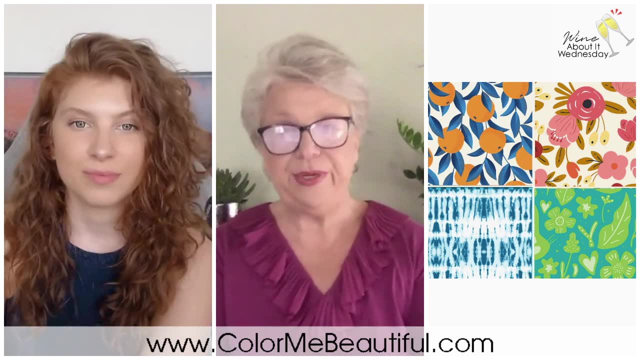 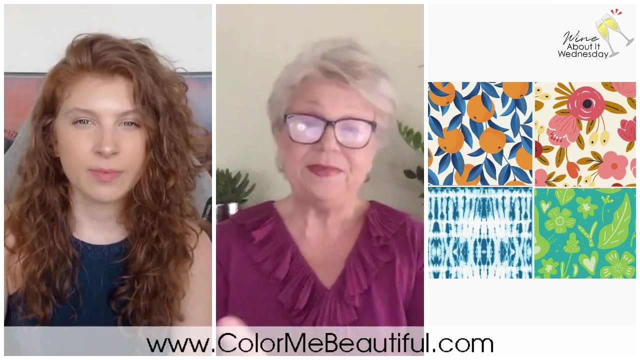 hand corner. um, and i pop that in because springs is a season of you get so many blues. for being a warm season, you just get to rock so many blues and i wanted to show something that shows that where you veer off from a true blue toward a teal, because that is lovely, all these patterns are gorgeous. so 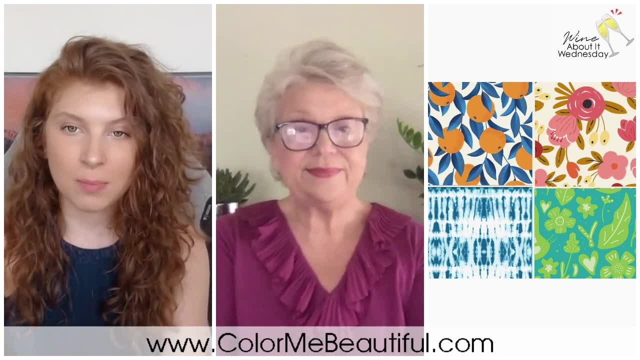 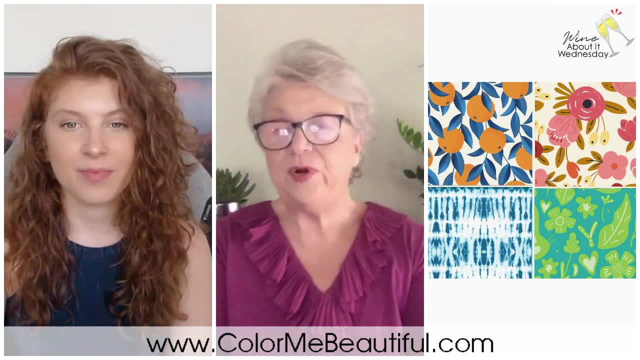 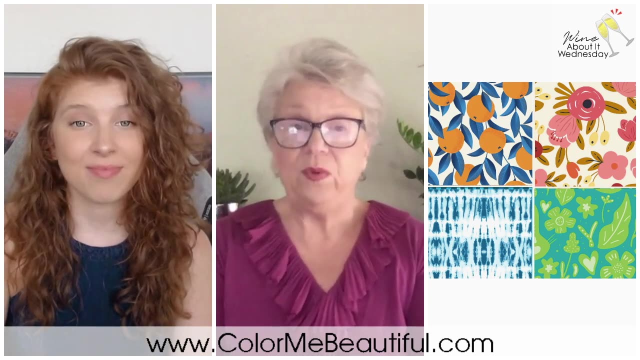 if you're a spring out there, just remember, look at these bright, bold patterns that are warm, that you can find in your color palette because, for example, springs, you guys are the only guys who get a light orange in your color palette. um, when sarah, when she goes for one, she has to move for a pumpkin. 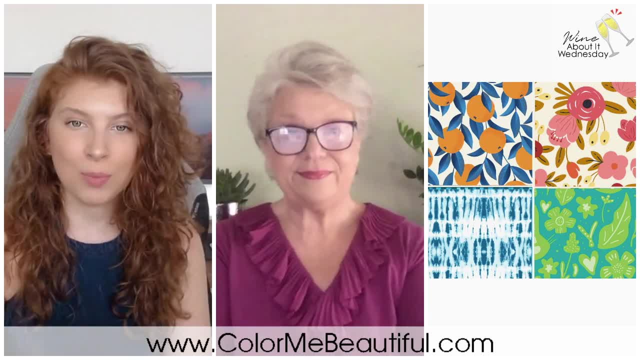 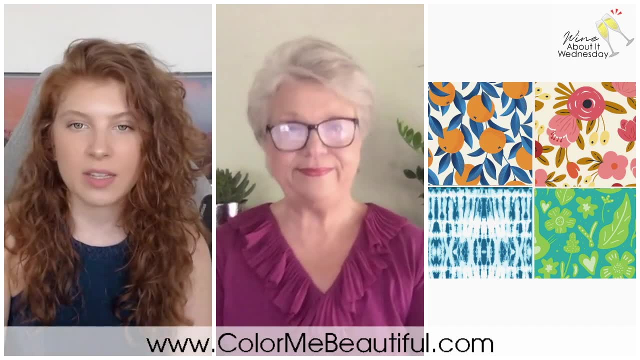 yeah, it definitely has to go deeper. so springs get that bold, bright orange and then autumns have to move a bit deeper to get more of that orange. so that's what we're going to talk about today. if you're into pink, plays colors, think green comes in. it'll be going to be your kind of. 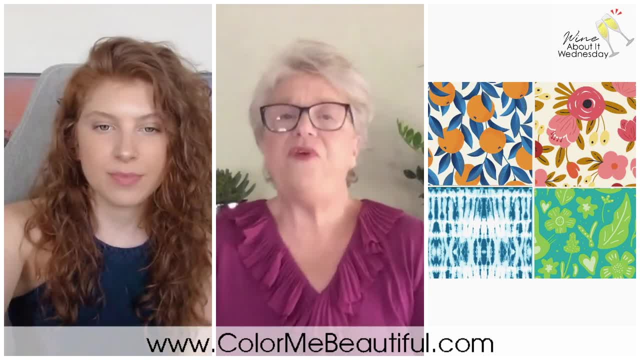 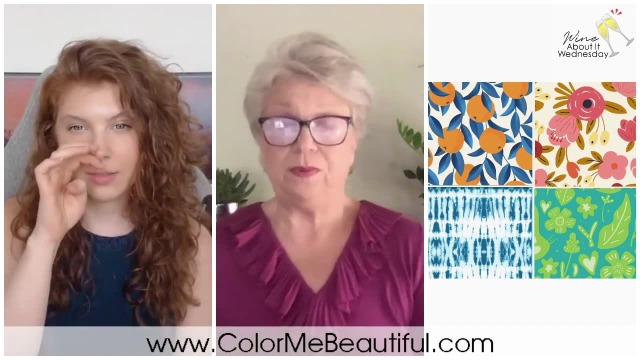 tho green color. if you are into these dark, então you know if any flowers- like i usually do, they goishENS- have to have a pretty overt pink on it. um, when you go out there, they have to give you a gradient of pink or helps with that sort of you want to get, with that sort of… and you 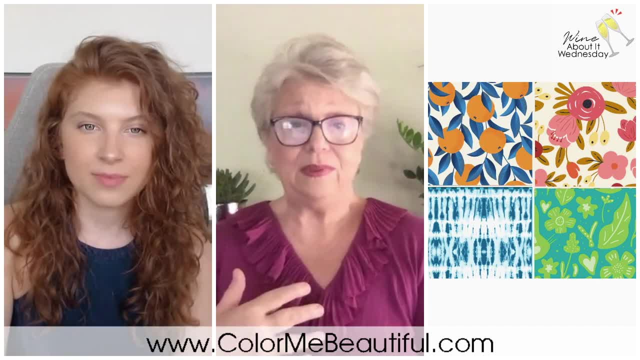 that's perfect mentality. you don't want to be looking at a olive or a black pink. i think your color palette is not your regular pink. you need to really work with resources and to recommend them so, and with the costumes you're able to use colors a lot better than with the. 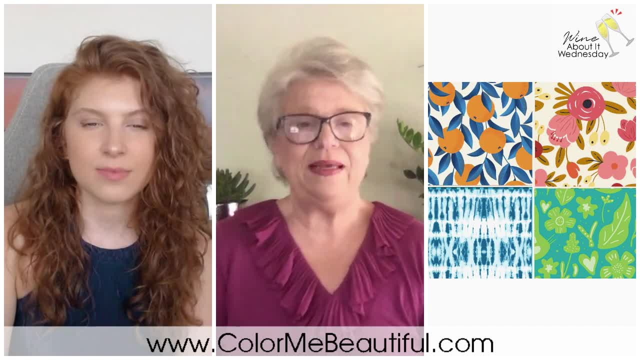 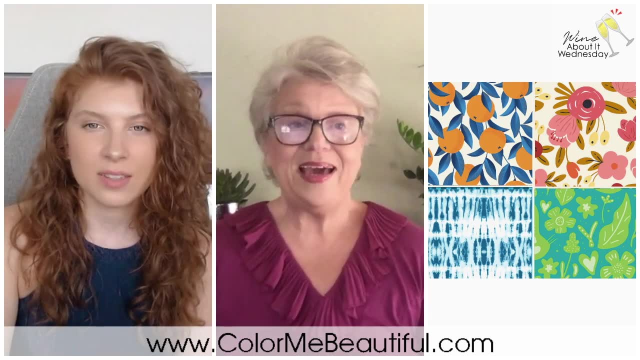 original. you just wanted dessert print on him our colors, but he's kind of a bicycle carrot. yeah, it's a comic like i will um the camera. i'll g vocal grid at his last here, price song winter. but you gotta have some friends and it's kind of friends that I was just 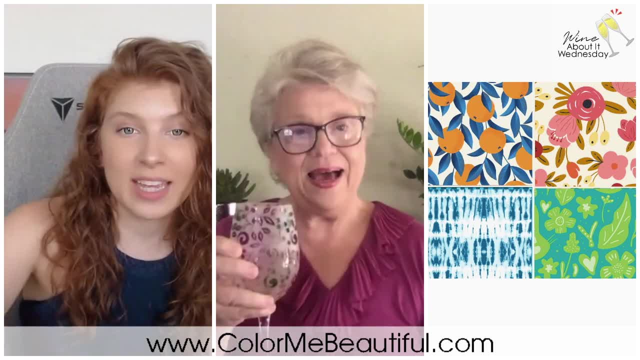 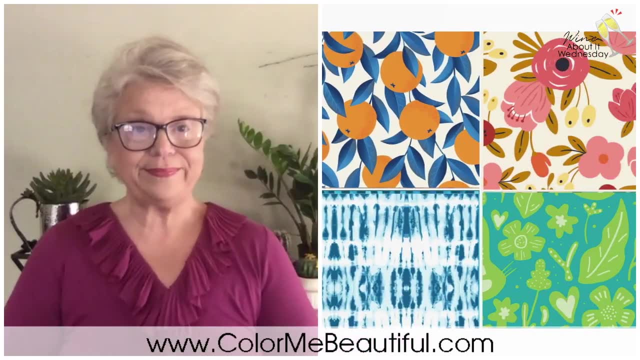 thinking it might be fun to bring up all four prints on the screen so everyone can get an idea. but can't you only do three? let's see we're about to find out. all right, then I get rid of me. I'm gonna grab the other warm season to show and. 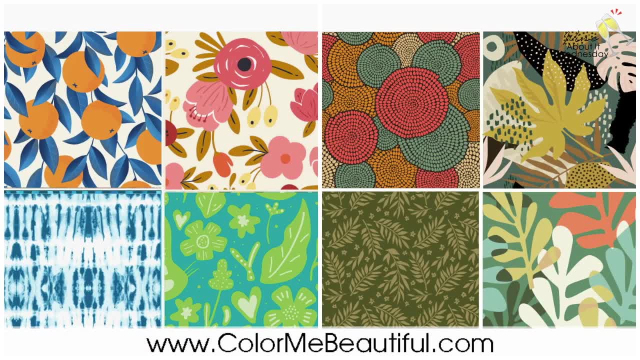 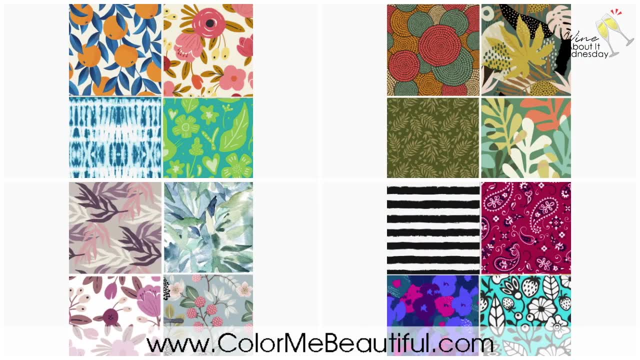 then I'm gonna get rid of you and then I'm gonna show our summer and then our winter. so on our top left we have our spring. on the top right we have autumn. on the bottom left we have summer. bottom right we have winter and the bottom 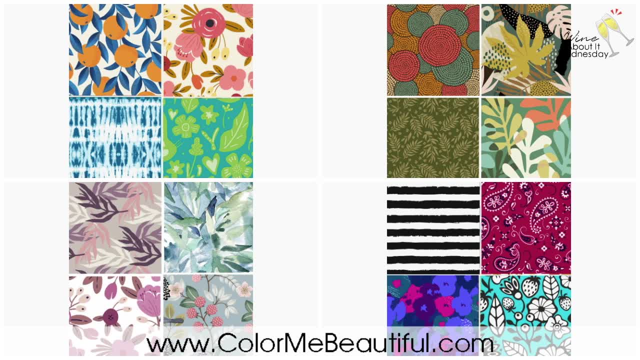 right, we have winter, all right. so now this is just kind of a quick look at all of them together so you can get an idea. but throw a question out to the audience and the question is based on your preferences for these patterns. would you be able to determine: 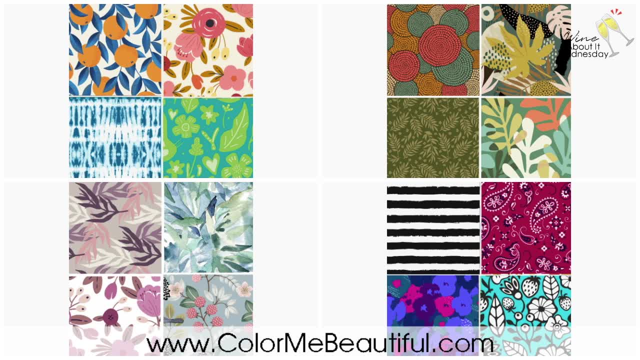 your season or someone season. I honestly, I am really loving the summer patterns, but I really so there's. I guess there's two in the summer that I really love: that blue green one and the one with the strawberries. Now, I think the strawberry one is just too cute, So that's the reason why I really love the strawberry one, But that blue 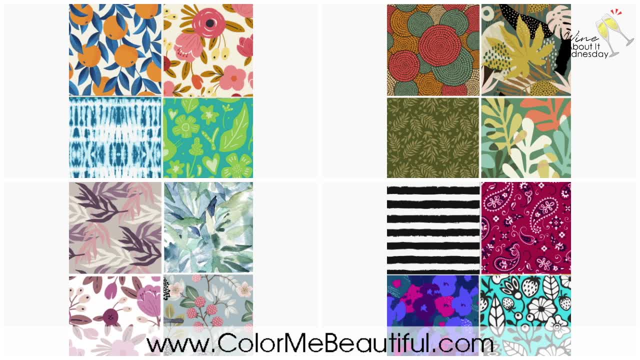 green pattern in the summer palette. it has to be one of my favorites. Granted, if I was going to get ready, I would probably do the top right in the autumn color, To be honest, like if I had to pick one to throw on the floor. that would be the color for me. Yeah, I would have put you in the 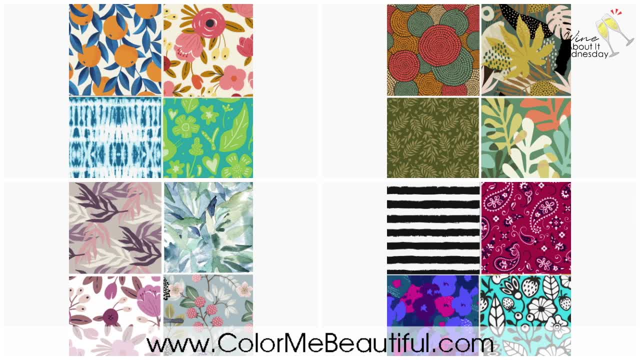 bottom, the bottom right of the autumn palette, I would wear a lipstick that orange, So I know you would. And now, if I was going to choose a pattern for you, though, I would either do the strawberry pattern that I love, probably because I think it's just so cute And I think it's awesome. 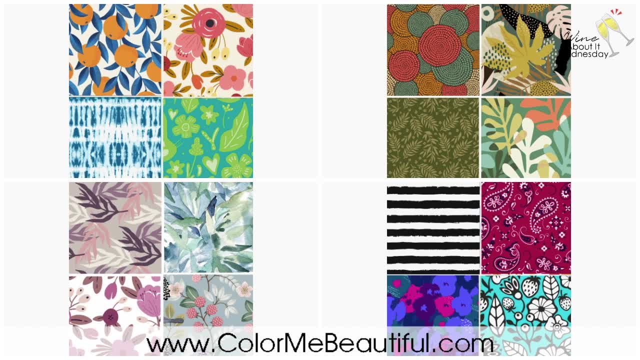 But also the summer, out of the summer square, the top left with the leaves. the purple, the pink, the light lavender, that like one color background that would look gorgeous on you. I love it, Love that. What we can do in a future video is- I'll take the one that you love so much with the 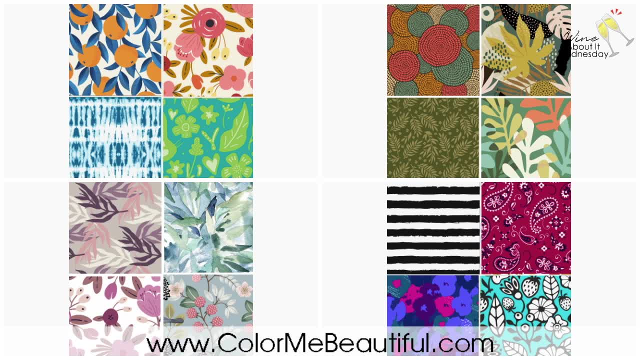 berries, and I will seasonalize that particular pattern and create a version for winter, a version for summer, a version for autumn and a version for spring, because nothing is more illustrative than seeing these kinds of things up against each other, Like, for example, what we: 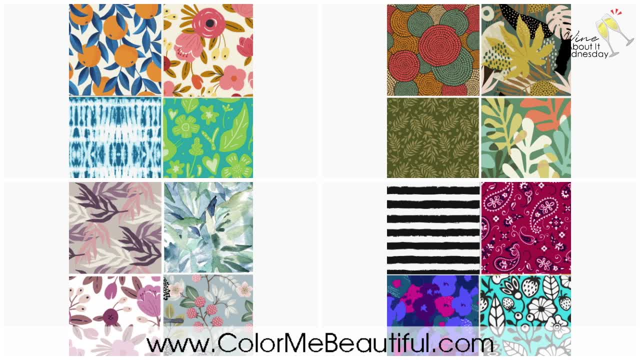 know is that there are two seasons that are the boldest of the seasons, two seasons that can pull a lot of contrast, And that's the spring and the winter, And they're two seasons that are softer in terms of their overall contrast, And that's the summer and the spring. And I think you 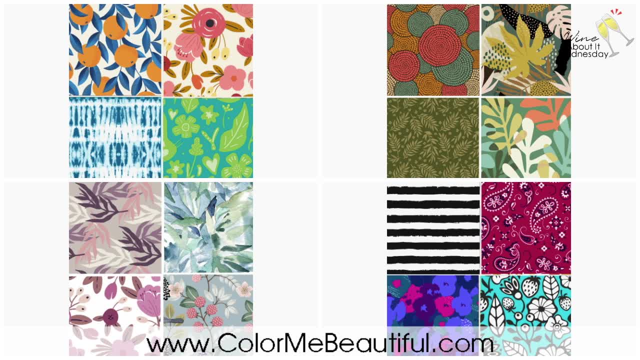 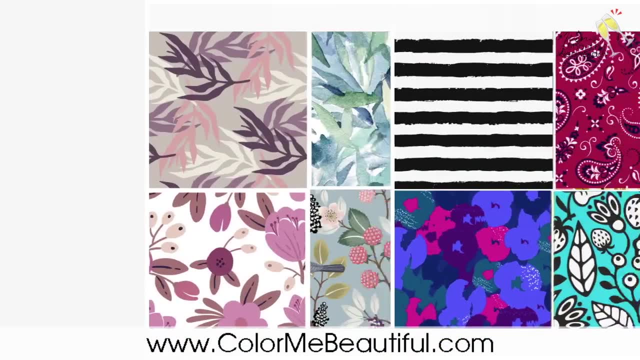 can see that here very easily. Quick correction: summer and autumn. You know I think I've been home too long because I got winter on a little while ago. Well, don't worry about it, because I do it all the time. Now what I wanted to do. 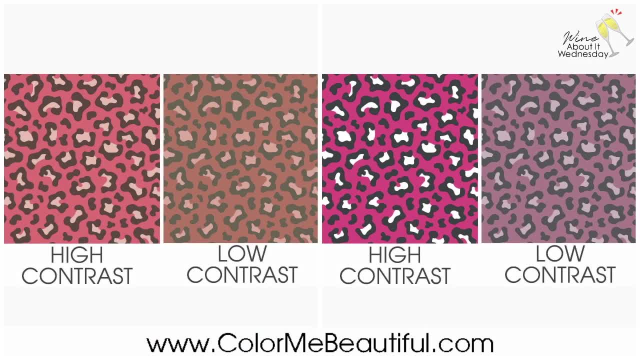 is: grab the high and the low contrast- So we can take a look at that as well- versus cool and warm. So on the left you have our two warm seasons And on the right you have our two cool seasons. Now 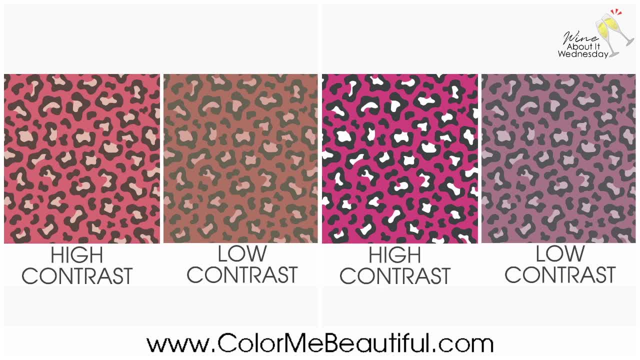 from left to right. we have spring, autumn, winter and then summer. Now could you choose your season based on your preference here? What looks the most like your wardrobe? Yes, I could absolutely do that. Being in autumn, I love, love, love that rust color. I. 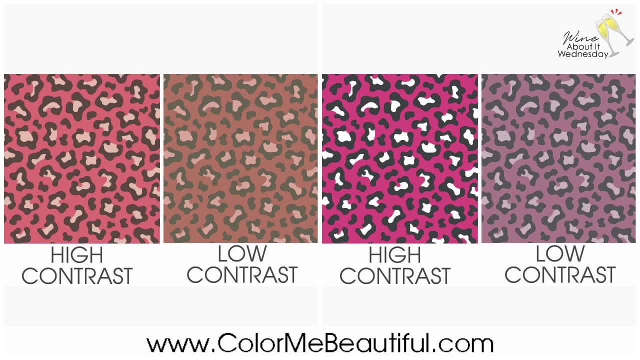 gravitate straight towards it. What about you? Well, yeah, I could, because anything that has a grayed out kind of that's grayed on the spectrum. it's almost like in my world: when I'm choosing color for myself, I look for something that has 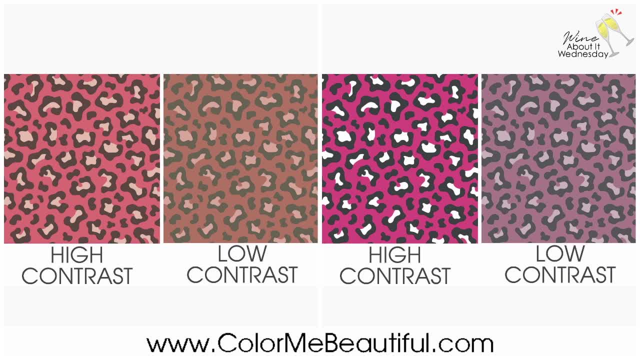 had a bit of adjusting of powder on it. you know, across the board something that's that where the vividness or the sharpness? in my case, if I were to wear that high contrast print, I would look washed out, I would look pale in comparison to that print, And so I look for something that's not going to swallow. 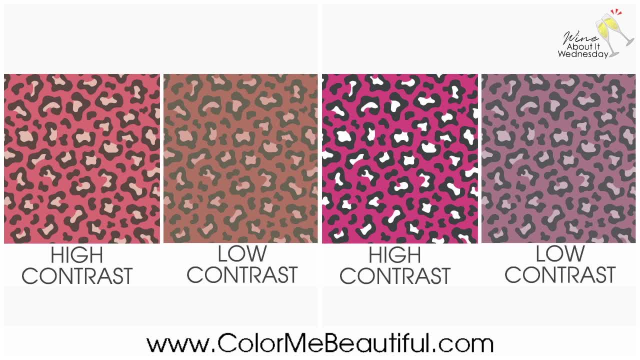 me up and make me look washed out. What about everyone watching? I'd love to hear if you gravitate towards your seasons print Or if you gravitate towards a different one, Yeah, And if you can tell us what your favorite print is. 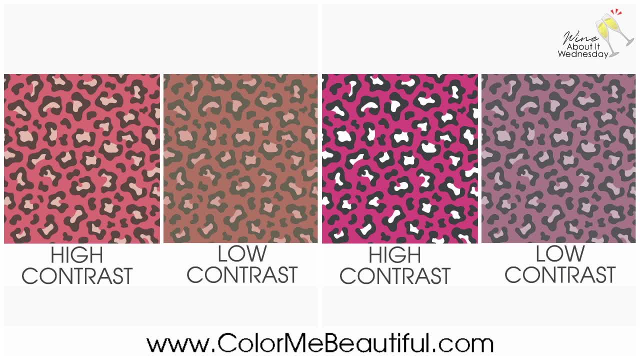 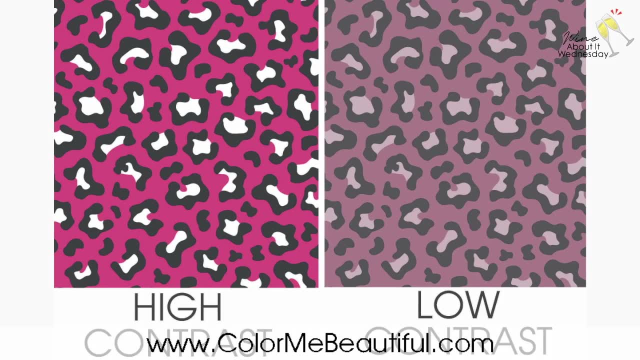 send us a picture. that could be fun too. yeah, I think we all tend to gravitate a little bit- I would say not a ton, but a little bit towards. we certainly know that we all make mistakes in terms of our palates and, like Lord knows, I've. 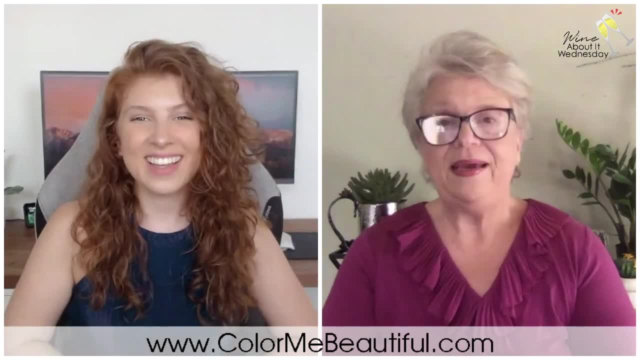 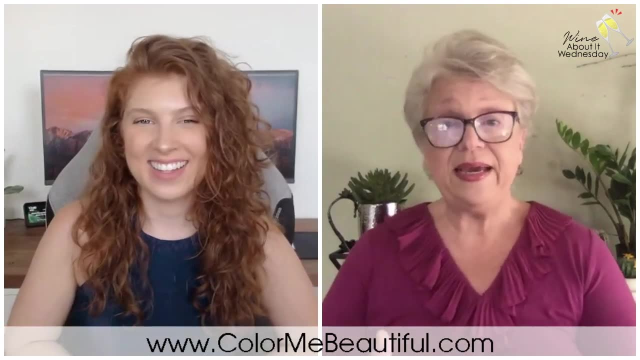 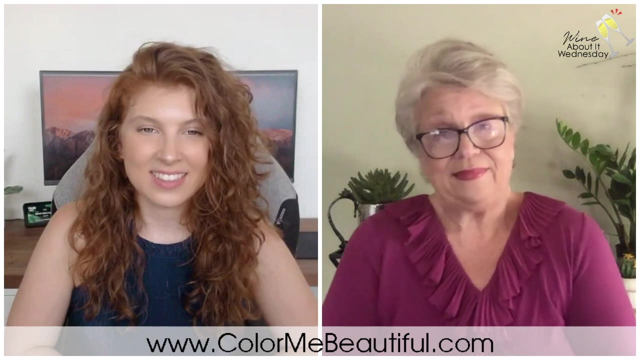 been doing a lot of cleaning out and, as you know, I'm seeing things that wear my closet and I was like- and I know better, it's not like I made that before I got the palette. you know, I know better and I did it and you know we all need to be. 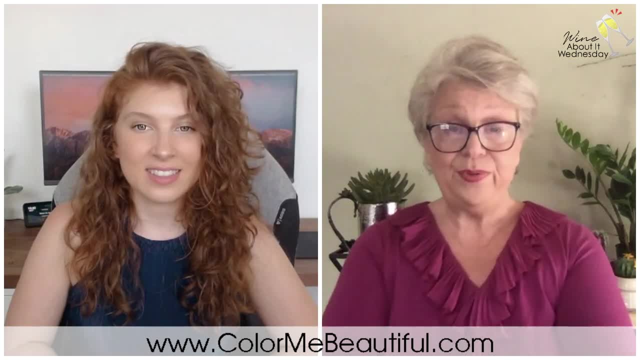 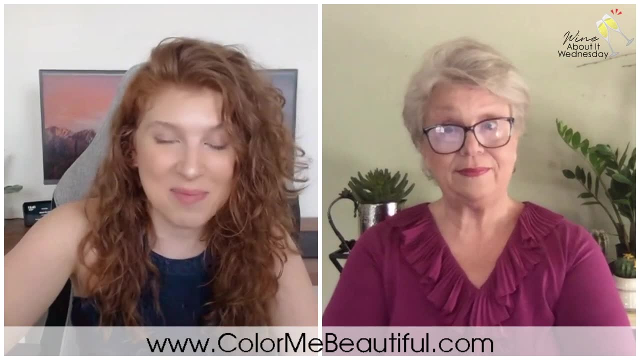 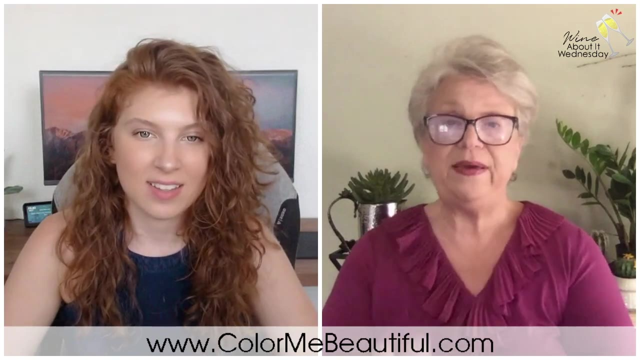 conscious of it, otherwise we'll end up with stuff we have to throw away. yeah, yeah, Koba has really made us clean out. okay, yeah, I got an interesting little perspective from the people- some of my the moms in our neighborhood. they talk. they were telling me that they've gone to the area thrift stores and we have. 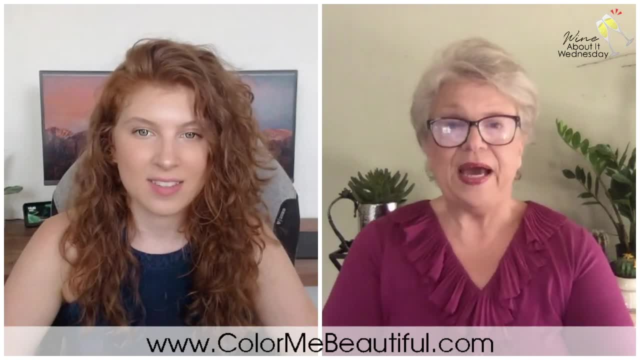 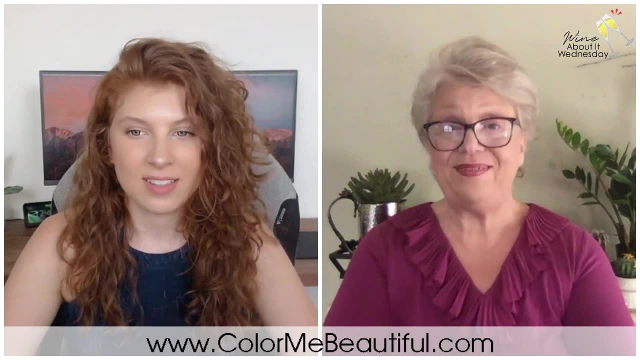 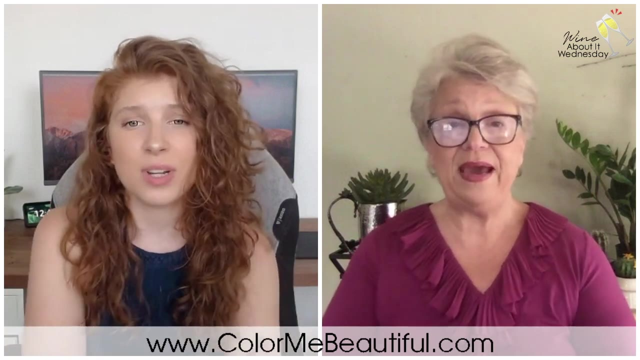 great thrift stores around here, which I love, and their donations are so backed up that they have container loads of them and some of them were just sitting outside in the rain and getting destroyed and because they- their donations, are so overwhelming right now, they haven't been able to manage them. oh. 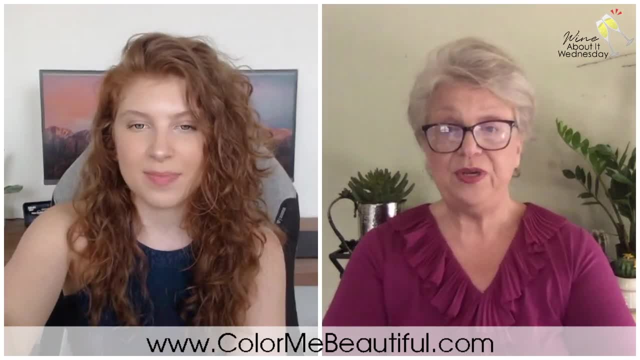 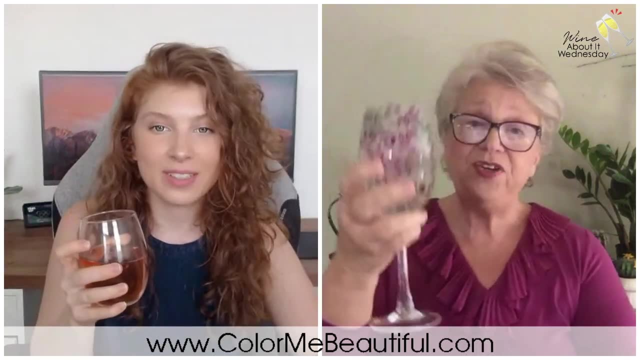 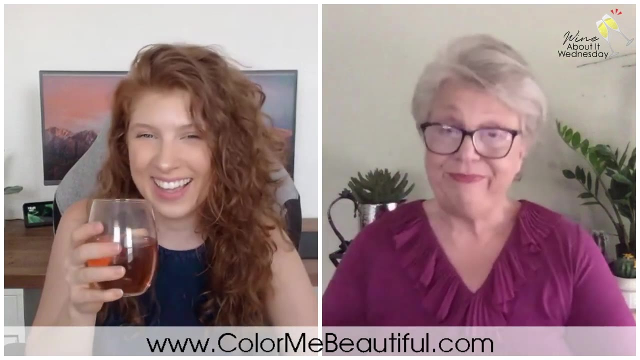 that's so hard to hear, oh man, especially since we love to recycle. yeah, that's too bad. well, sad to hear that. but new donations. I know, now the end of COVID-19. now I need to stop cleaning up my house. apparently you gotta get a storage unit until your. 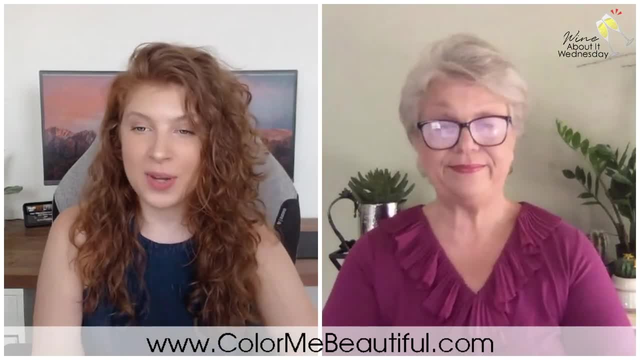 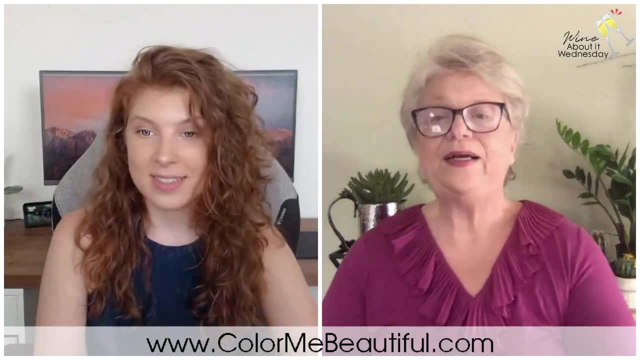 donations can be meaningful, true, so I do have a. let's see a couple comments. so you're in autumn, but you like the high contrast? hey, well, you saw that in your autumn palette. it's a little. we call it a soft season, but you can pull off a. 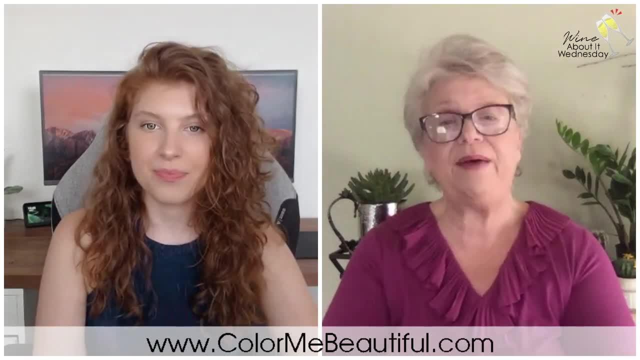 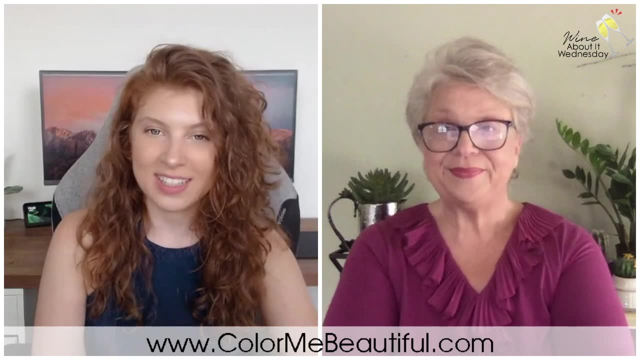 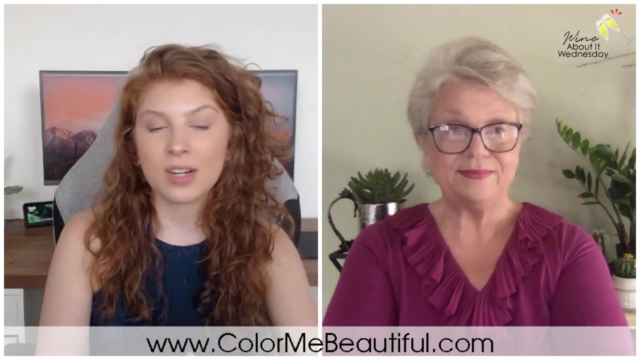 little bit more contrast than a spring. I mean, I'm sorry then I saw right. and then Cher towards her own. yeah, we always tend to lean a little towards the colors that happen to be in our palette and, honestly, sometimes if we're having a hard time, like doing color analysis online and just talking to people if they can't. 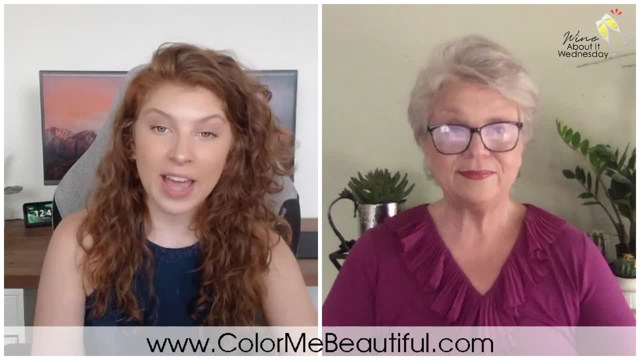 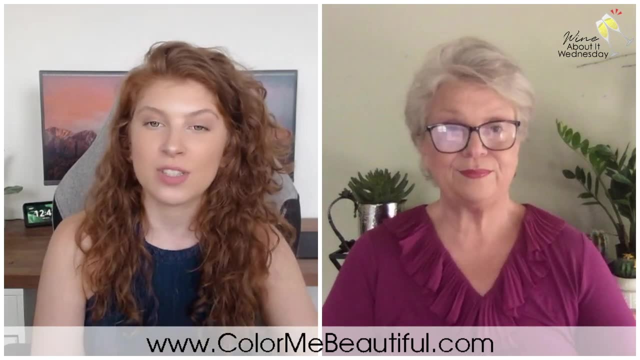 send us an image or something along those lines. one of the questions that we ask is: you know what are your favorite colors, what do you gravitate towards? and people, a lot of the time they don't know where they're going to put their colors, tend to gravitate towards their season. they just weren't able to put all of the 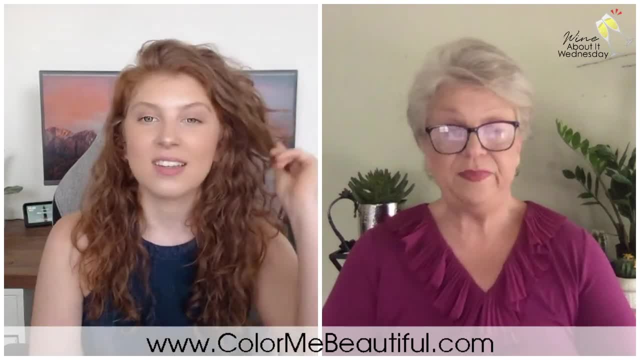 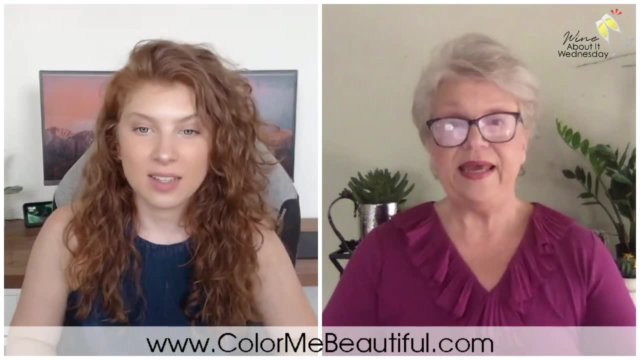 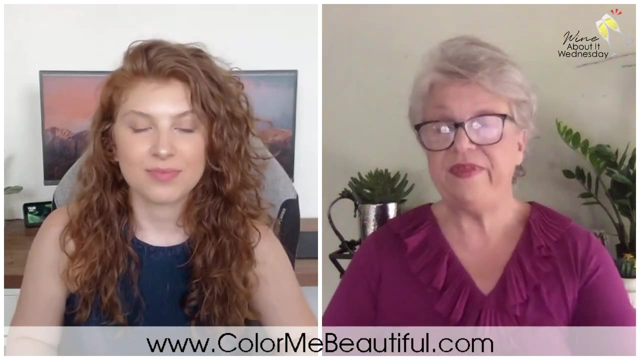 pieces together and we also last our last video we did for you guys. if you look, last Wednesday we did tiebreakers, certain colors in every season that only that people in that season can rock, can you know, look gorgeous in. and one of them that I always like this row out there for people who don't know if 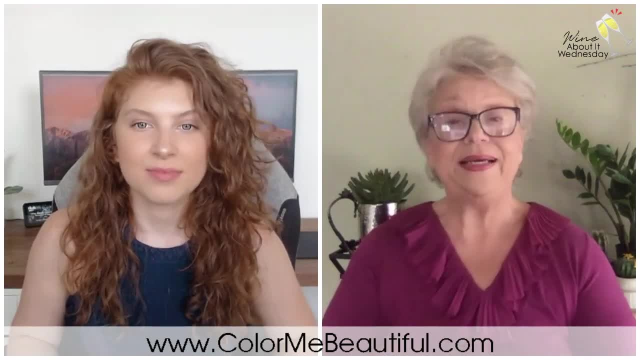 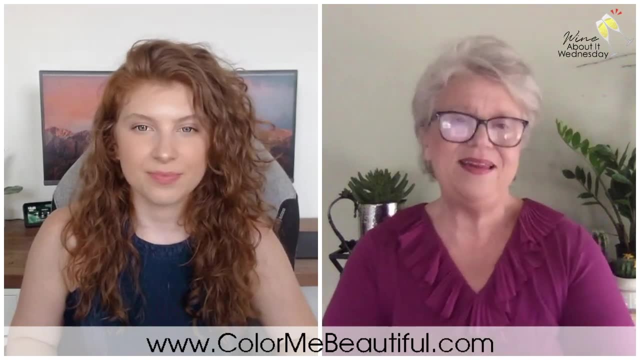 they're an autumn or spring, they say, oh, do you have red or blue highlights in here? and they'll say yes. and then I'll say, well, is your hair dark on the dark side or is it light blondish? and they say, it's not really either, and and so 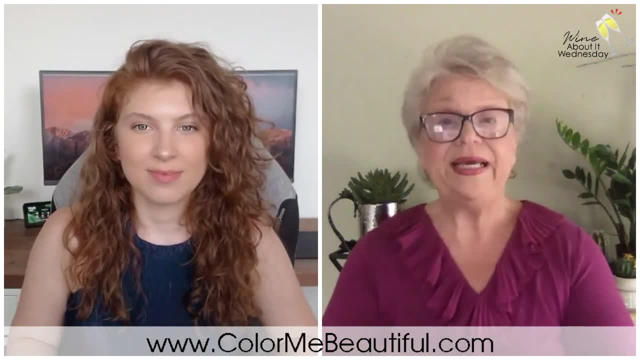 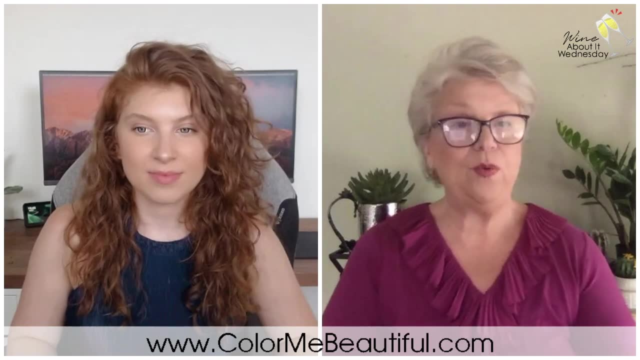 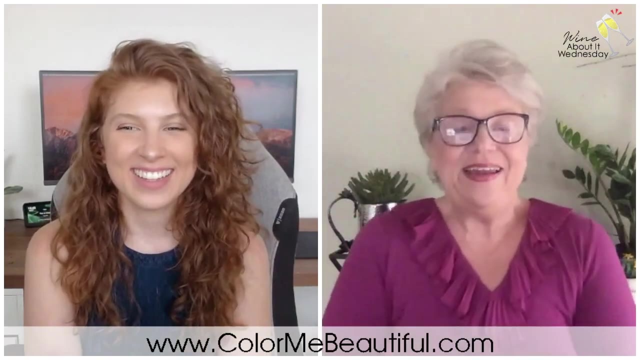 they don't give us any clues there and I always throw out the olive. can you wear olive? mm-hmm, it's. it always works, because the rare people who can wear olive are what I am and um, and the same is true with the people who don't know what they're wearing, and the same is true with the. 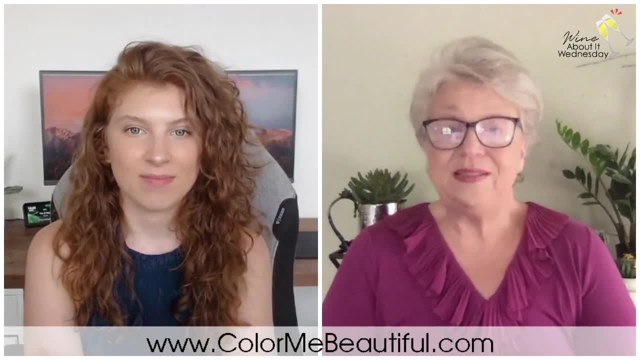 people who don't know what they're wearing, and the same is true with the people who don't know what they're wearing, and the same is true with the. you know the as a tiebreaker between winters and summers. you know whether they can wear the light gray and, and inevitably, winters are like oh no, it's. 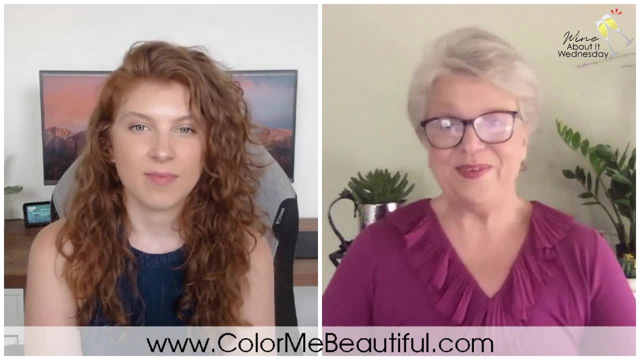 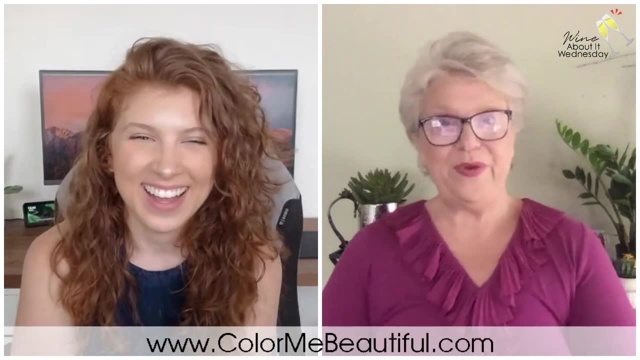 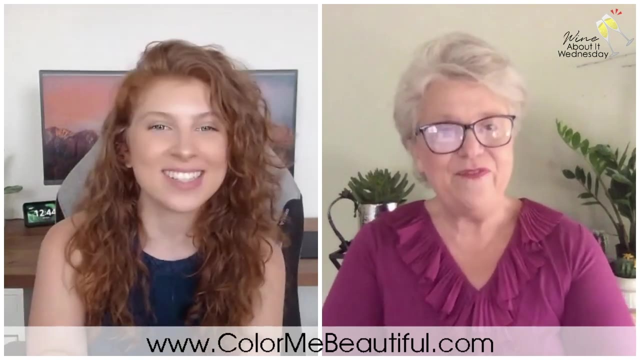 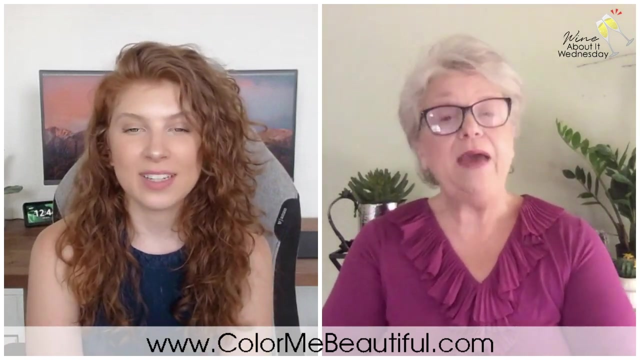 just come a grab on me. and then the summers get mad, love it. and then the autumns are like: oh you keep your gray. yeah, enjoy that gray. I'm gonna enjoy my mustering at my greens and my right three. a room in your home is gray. well, i haven't. i haven't painted yet. so and what color did you paint your bedroom? i um. 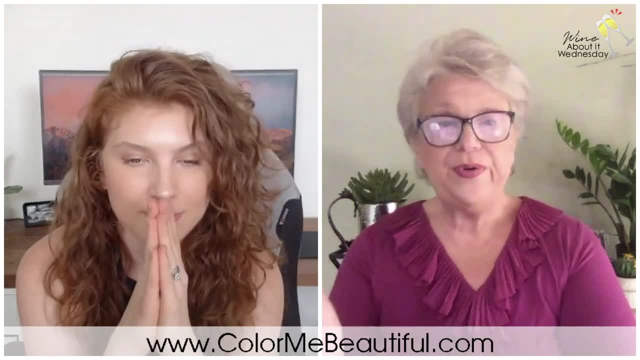 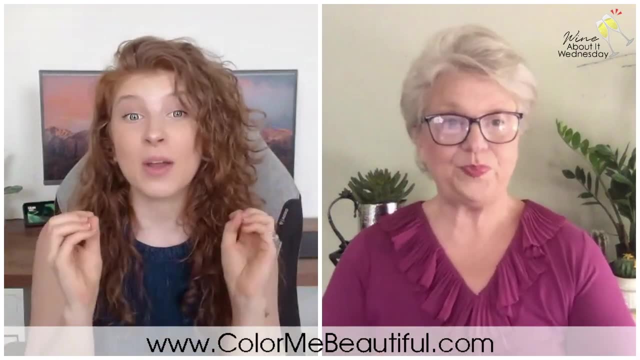 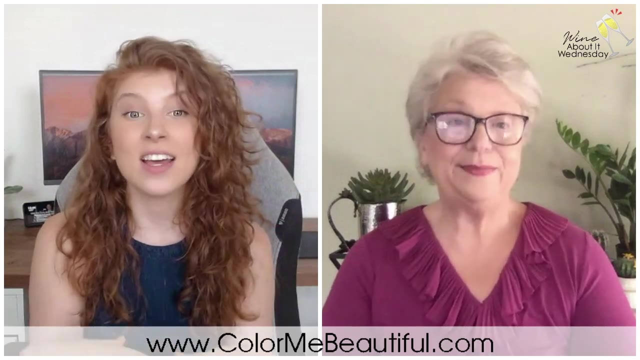 i did. what color is it, sherwin-williams? um, no, it's warmer than repose. it was right, it's great, it's gray, but it's a very warm gray. it's about as warm as you can get to and gray, it's what. agreeable gray. that's what it is. it's agreeable gray and it has you know if you want to take a. 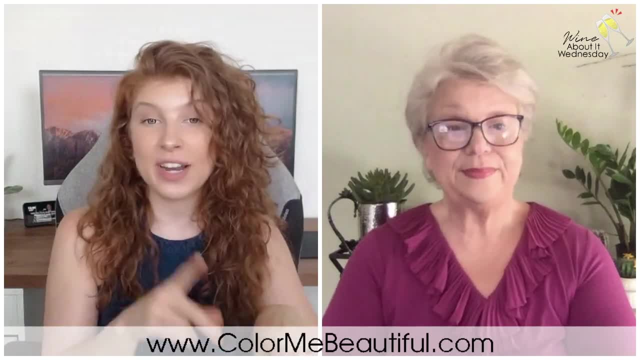 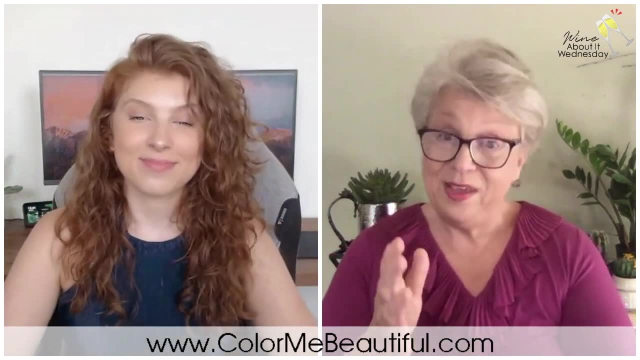 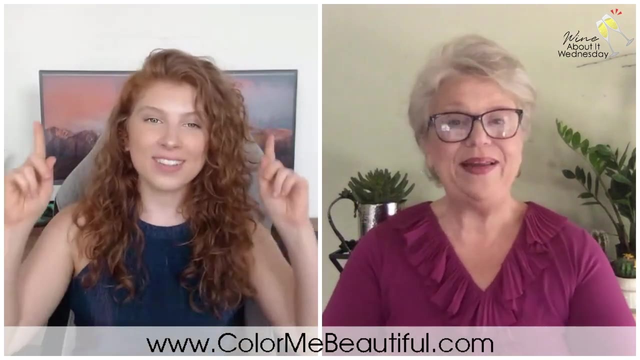 look at a warm versus a cool kind of gray, look at agreeable gray versus proposed gray, and one is a bit cooler and one's a bit warmer. so, but i will just repeat what i said before. you so rudely contradicted me: every room in your house is gray and the one feature wall that you have is blue. 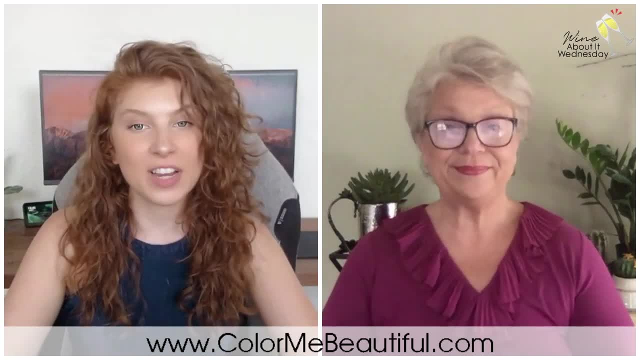 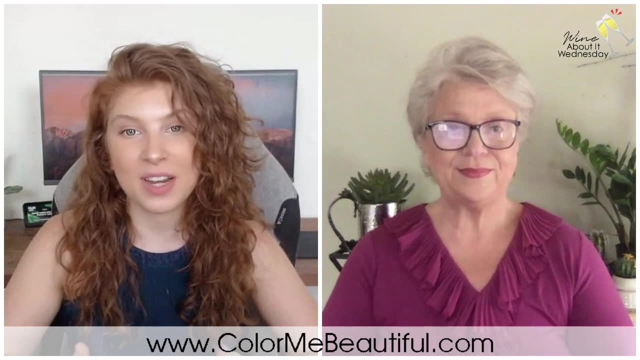 yep, i do have, and it's a cool blue. it's not a warm blue, it's a very cool blue blue. i have a lot of. well, i guess my green in my living room is a very warm green, so it's it's getting a bit. 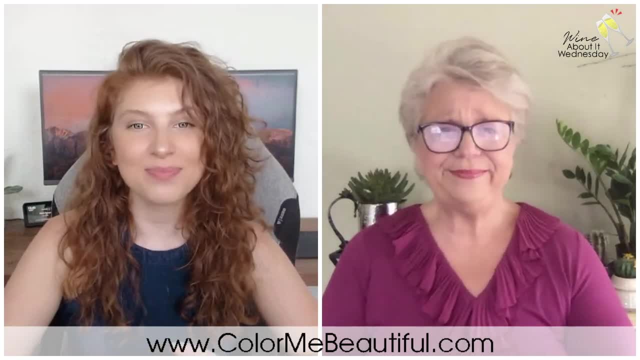 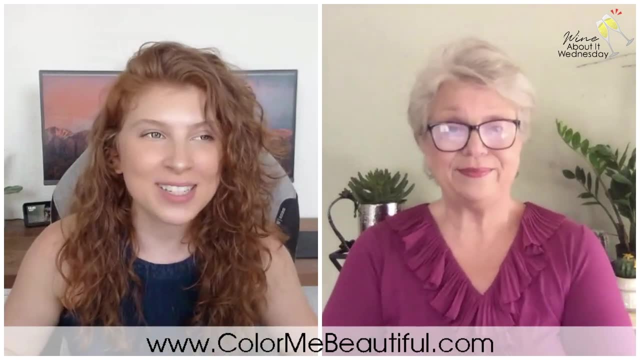 warmer in my living room. i am warming up. i would say so, don't be distant on my gray. i'm just saying if, beige, like if, or rust. if i could paint my entire house or rust or green, i would it. just it's too dark for that. 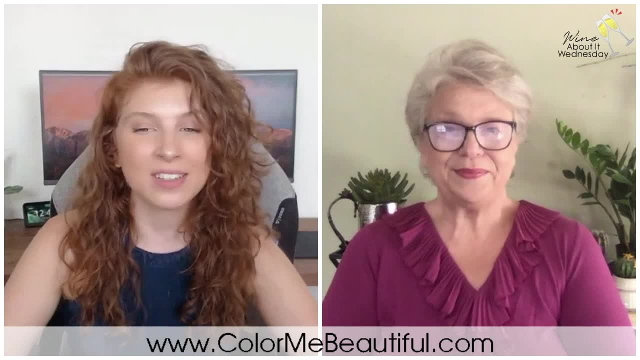 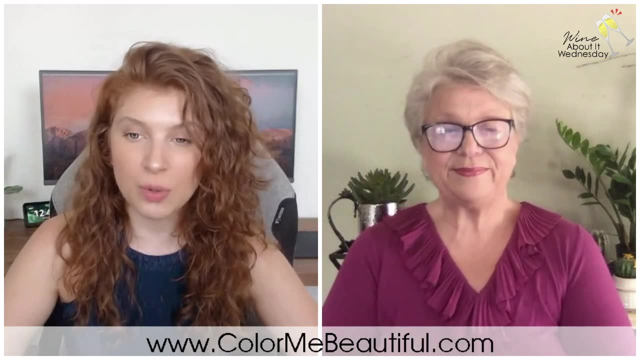 all right. so if anyone has any questions out there of patterns or high contrast versus low contrast, we'll make sure you get them all. yep, we'll send all of these images towards you. you can also comment down below. if you want to know what your season is, feel free to send us a message. 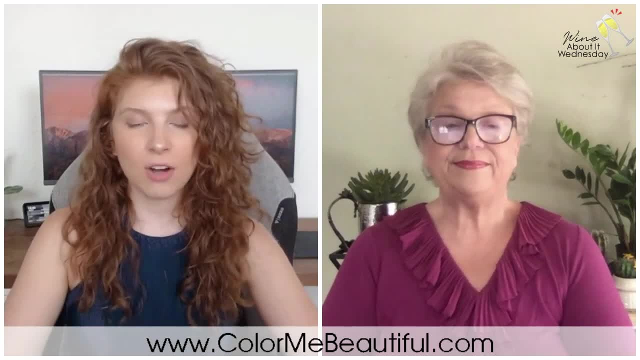 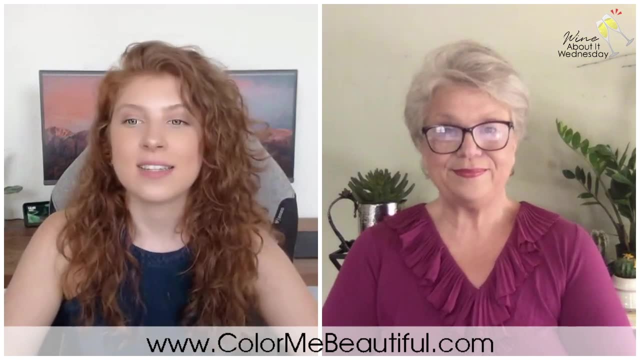 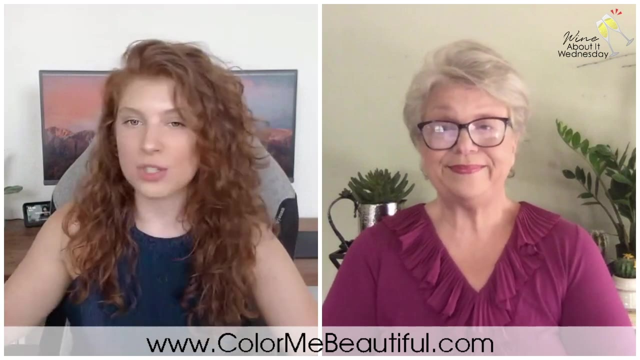 and send us an image in natural lighting of yourself. we do have to see you in natural lighting. um, you can send that on over. we'd be happy to help, and um, i guess that's everything. yeah, just let us know. if you guys have any other questions, we'd be happy to help you out. 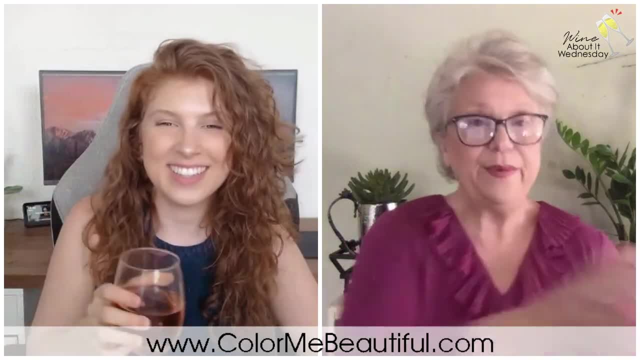 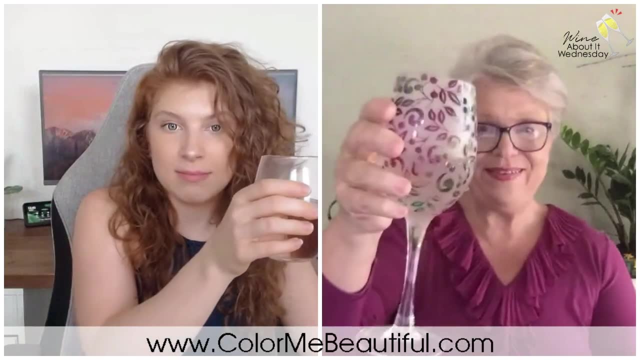 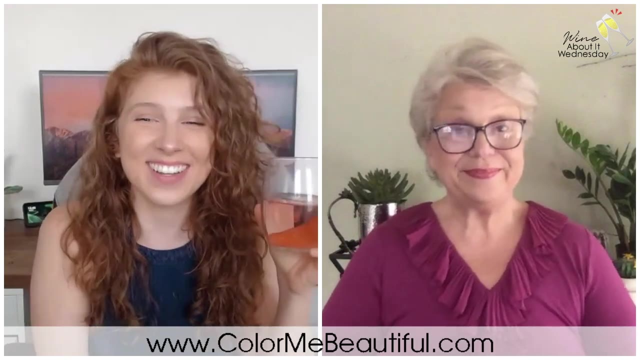 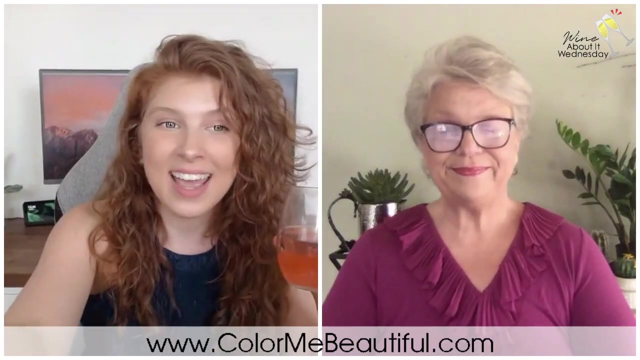 but i'm going to grab my wine, finish drinking now. we're leaving lunch break, yeah, so cheers, okay. oh, i know you're still going all right, so we'll see everyone on monday, for it's a beautiful monday. so have a fabulous weekend and we'll talk to you later.